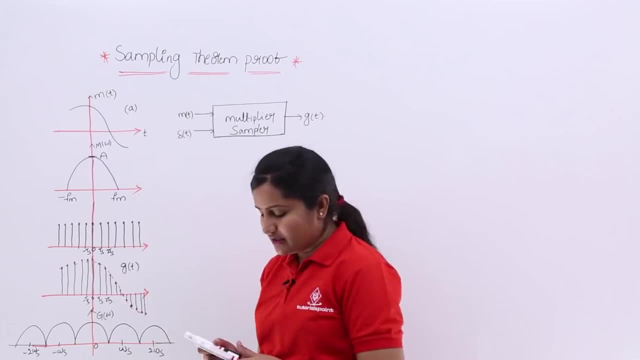 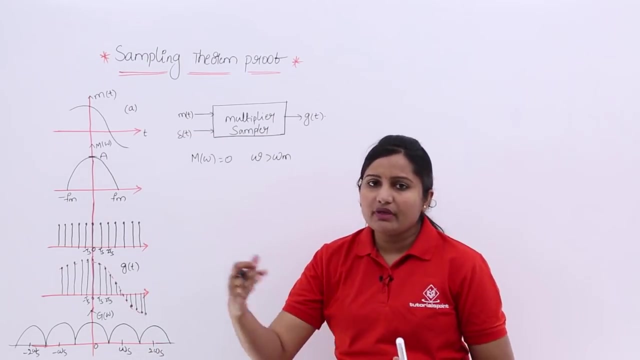 if you consider any transform of that message signal that transform must be m of omega must be 0 if omega is greater than omega m or f is greater than omega m. So that is band limited to fm means. beyond that there would not be any frequency components if you. 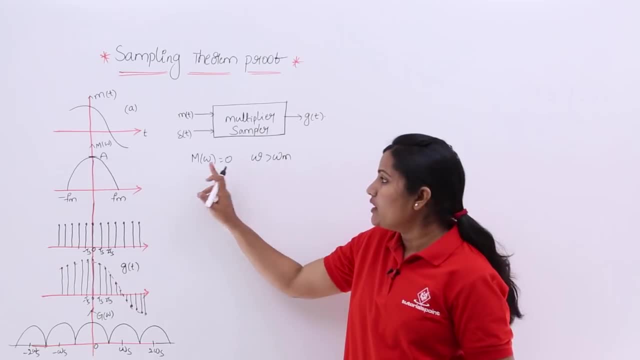 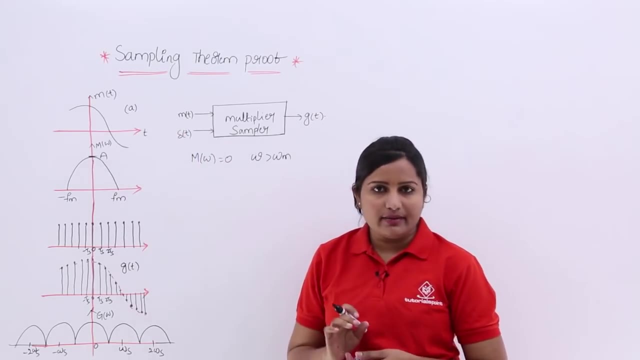 consider beyond that. that means greater than omega m. your transform must be is equivalent to 0. that is nothing but band limited signal. So I am considering a continuous signal m of t which is band limited to fm. the meaning of band limited is, if you consider: 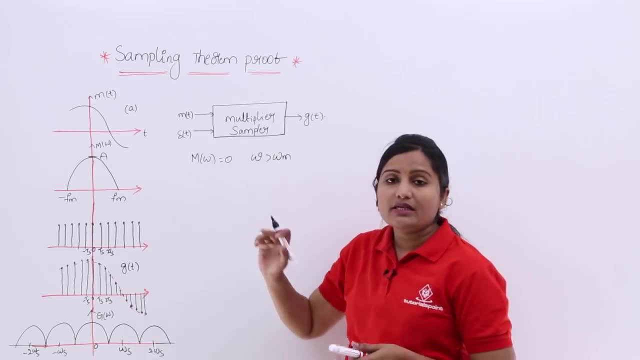 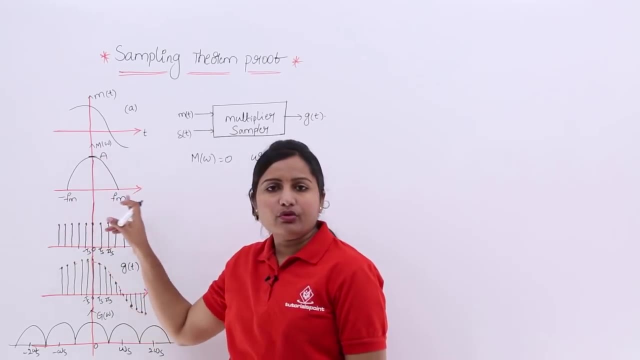 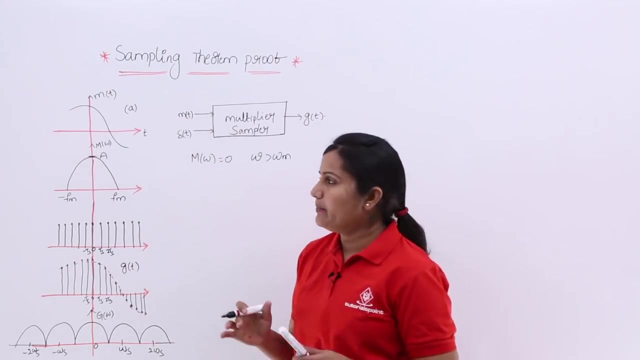 greater than omega, m or fm. your spectrum must be 0. you are not having spectrum beyond fm. You can see my spectrum is band limited to fm both sides. If this is the spectrum of your message signal m of t, then how you will get sampled signal means we need to consider a sampler or multiplier. 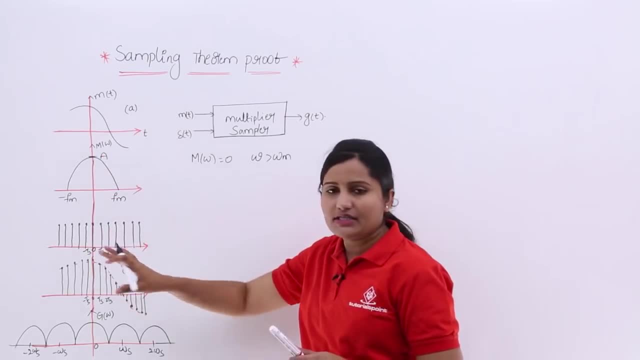 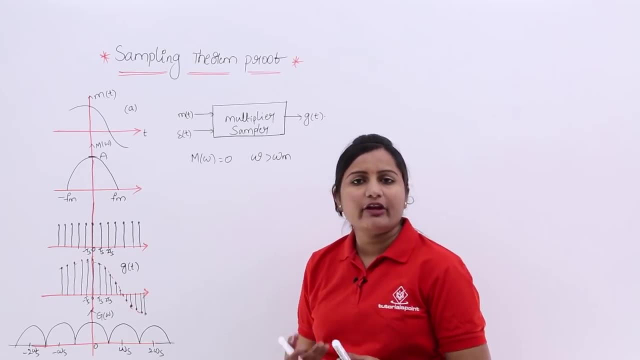 which multiplies your continuous signal with a message string, with a pulse string. This pulse string is having time to be sampled. So this pulse string is having time to be sampled. So then, what is the sample frequency? So the sample frequency is: there is a time. 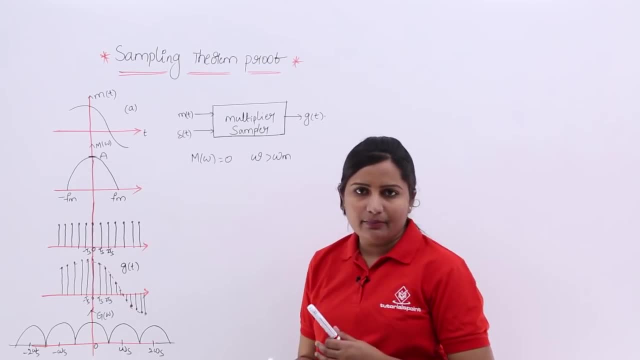 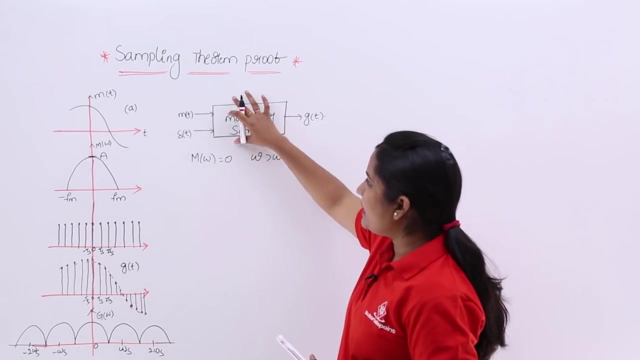 period- ts, that is nothing but frequency- as fs, sampling frequency or sampling time period that this need to maintain. So here I consider the sampling time period as ts and obviously the sampling frequency will be fs. That means 1 by ts. So here, just by multiplying this pulse, 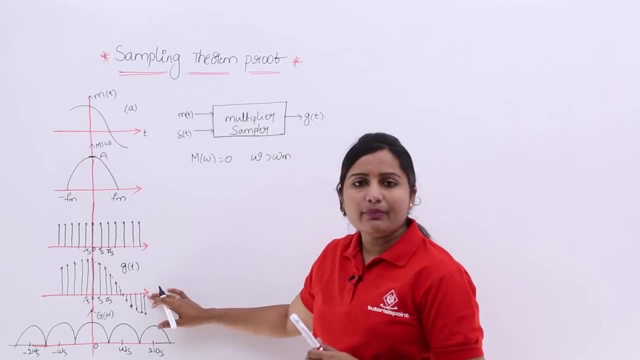 string with m of t, you are going to get your sampled signal. this is your sampled signal. I named it as g of t for my sensing. So how you get your sampled signal. this is that q of t. So my convenience for ah derivation purpose. i named it as i labeled it, as g of t. so here you can see. 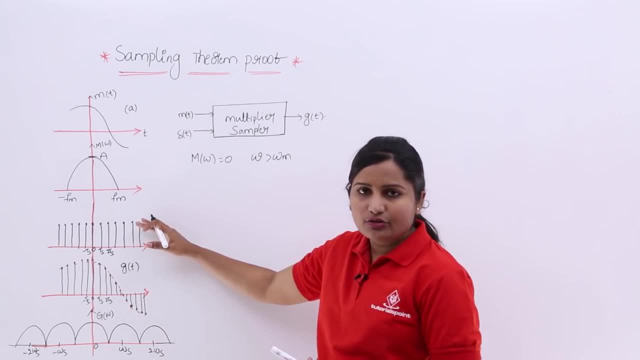 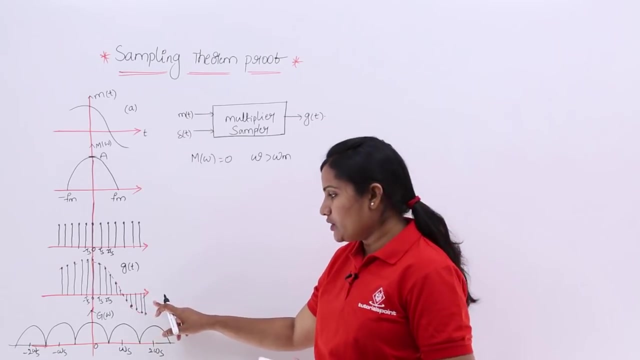 as i considered fs greater than as equivalent to 2 fm. so as i consider less time period, more frequency as sampling frequency, i am getting my actual structure of message signal in sampled version or a discrete version also. so here you can see by observing your sampled or a discrete. 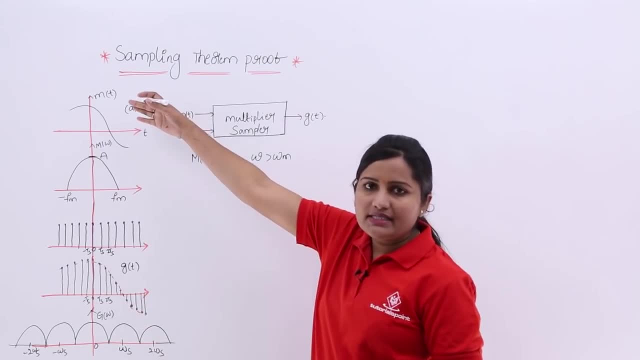 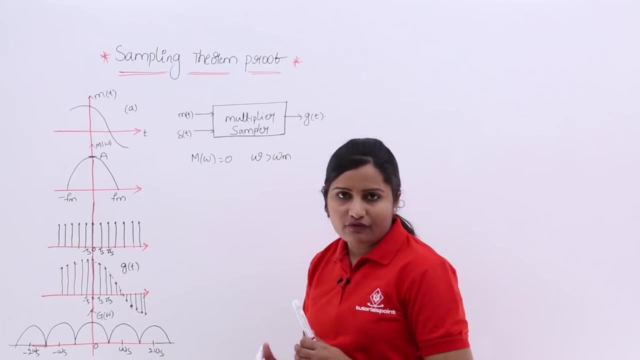 version of signal itself, you can say what is the actual message signal. so here i am having spectrum of this sampled signal that is considered as g of omega. i am going to derive the equation for g of omega now, so that g of omega can be used for reconstruction purpose. so now you can see. 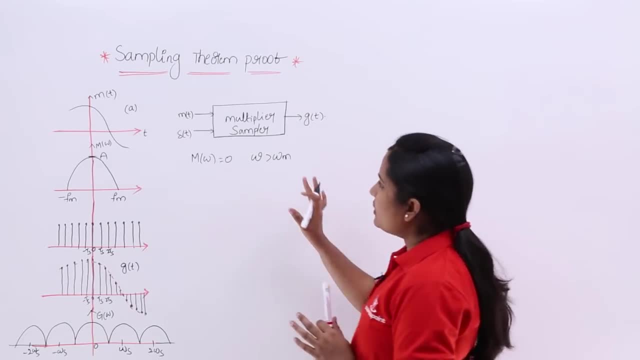 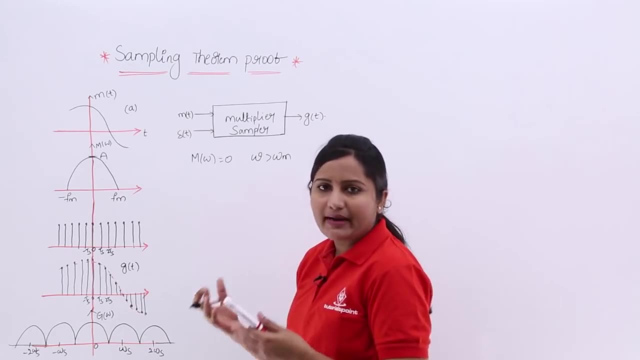 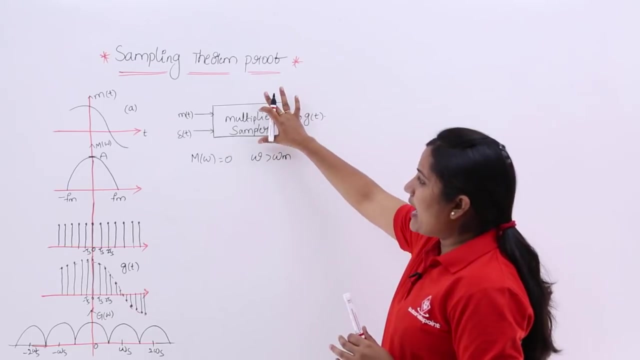 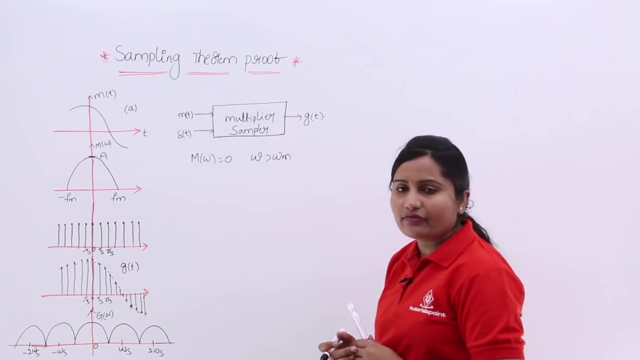 how i will take this. so here i just want to consider the equation of sampled signal and spectrum of sample signal. that's it. i want to consider the sample spectrum. so here, if you observe, so i am sampling process. sampler will do just multiplication, multiplication of your message and del of t. before multiplying, i want to consider a value for my impulse time. del of t. 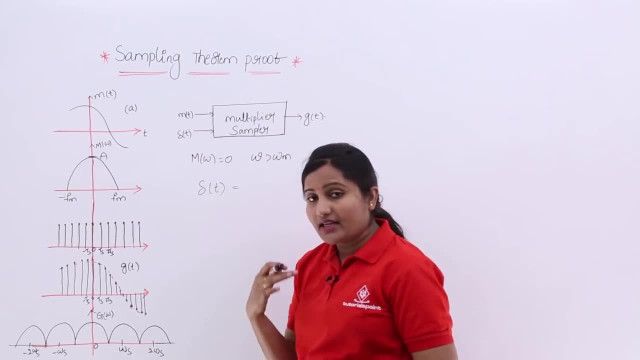 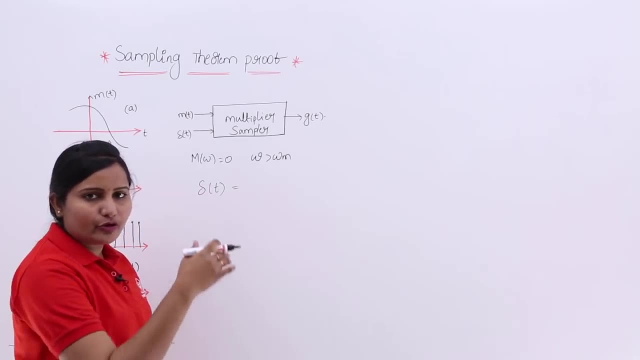 so how i can represent any impulse time means again i am getting into fourier series representation. how i can give fourier series representation for this del of t means i am going to use trigonometric fourier series. so here i can give any signal you can equate with. 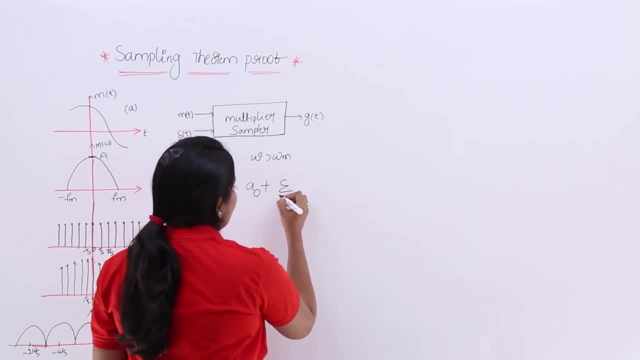 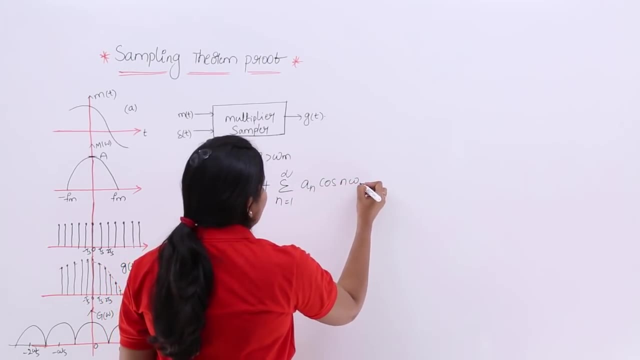 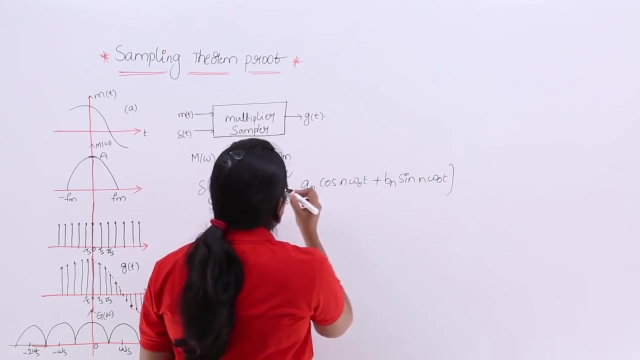 trigonometric fourier series, like a naught plus summation n is equaling to 1 to infinity. a n cos n omega naught t plus b n sin n omega naught t. this is your fourier series representation for this del of t. so i am going to use trigonometric fourier series. 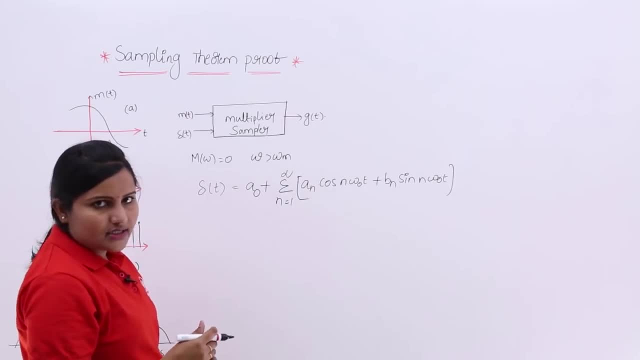 representation of your trigonometric fourier series, representation of del of t. so how we will get trigonometric series representation means: first we need to equate with standard equation and we need to find out a naught, a, n, b, n values and we need to substitute in this: 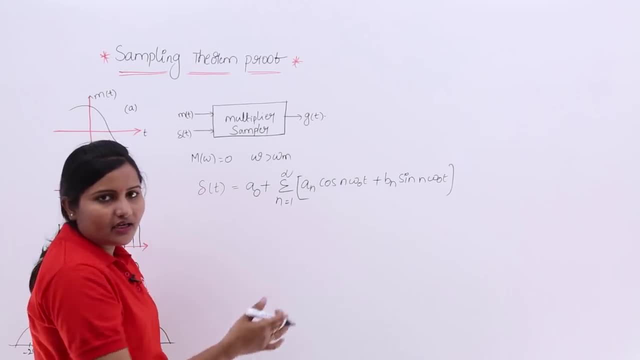 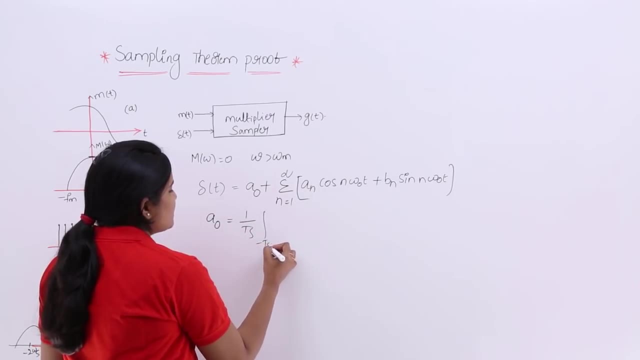 to get actual representation of your del of t in trigonometric fourier series. then what is the value? of a naught means? so 1 by t s, integral minus t s by 2 to t s by 2. so here you are having del of t d t. your function is del of t d t. this is your a naught value. 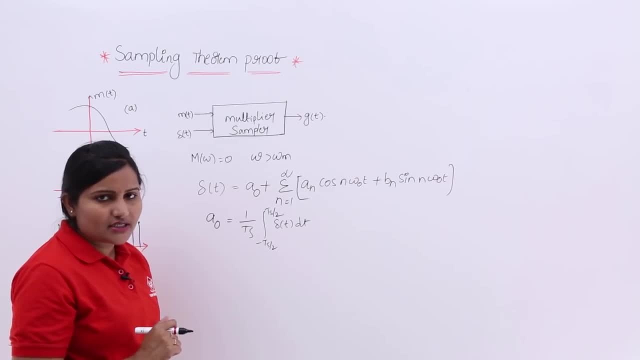 please refer fourier series representation, trigonometric fourier series representation to get all these reference. so here if you want to find out a naught, you need to consider: this is standard formula: 1 by t s, integral t, t by 2 to t by 2. whatever the limits you 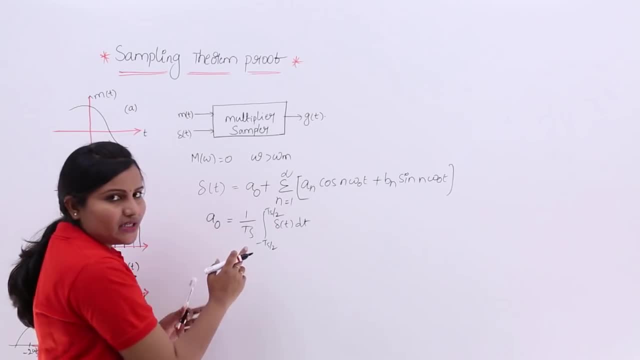 are taking so del of t d t why i consider t s means my time period of my signal, time period of my signal, which i am going represent with trigonometric fourier series. it is having t s time period, so 1 by t s. i tegral t s by 2 to t s by 2 my signal t, t will give you. 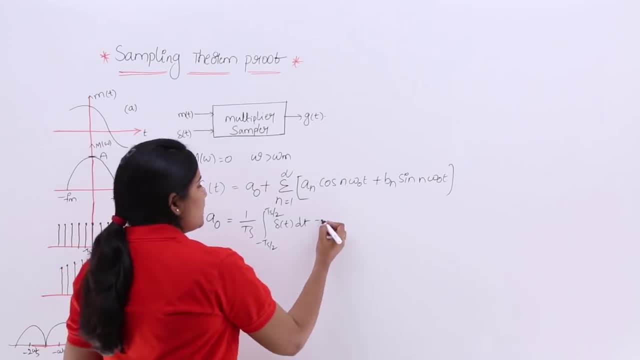 d, c, component or constant in the series. so this is equivalent to, as i told you when you saw impulse function in any integration, no need to integrate. you can write like like this: why? because del function is only having value at del of 0. so you have to write this: 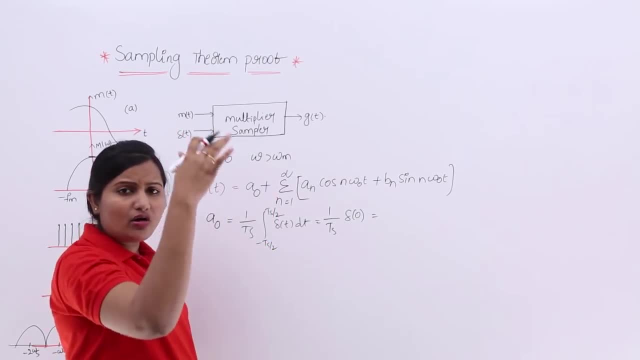 only so. these are the measurements here, how we are going to take it here. this was one step of og最breaking Maya. when you will have efficient chiang maga. thank you see, if 0- no need to integrate all the time periods, Just at t- is equal to 0, you are having value. 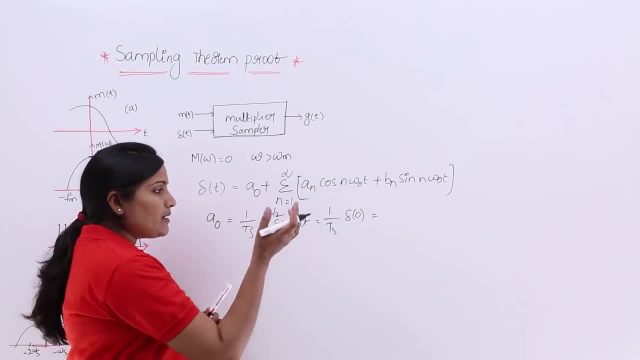 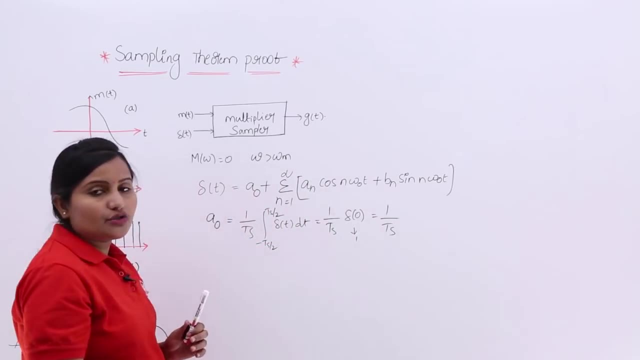 in all other cases you are not having value. So I am just considering this value. then I can write del of 0 as 1.. So 1 by t s into 1, you are going to get 1 by t s. So now coming. 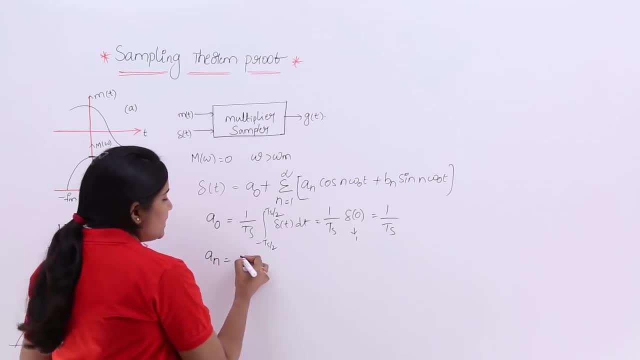 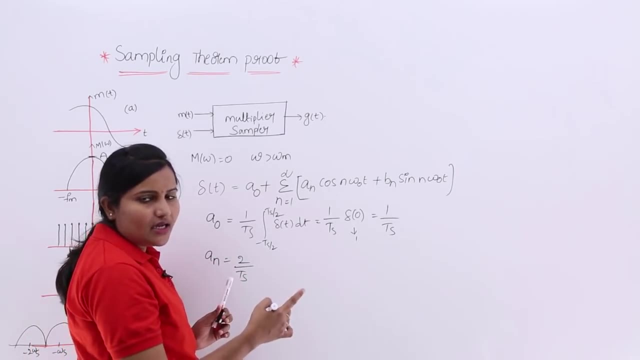 to a n. if you want a n equation, that standard equation is 1 by t s or 2 by t, 2 by t s. I am writing t s in place of t in standard equation. that will be t why I am writing t s means. 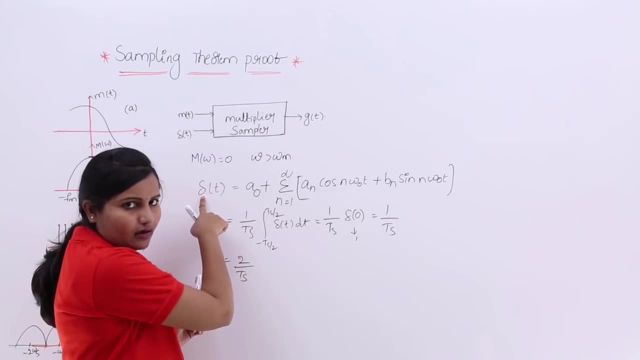 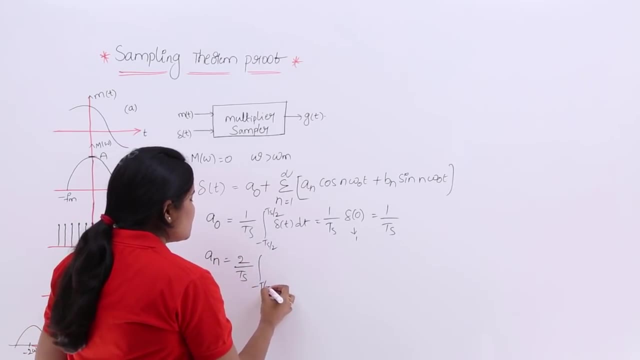 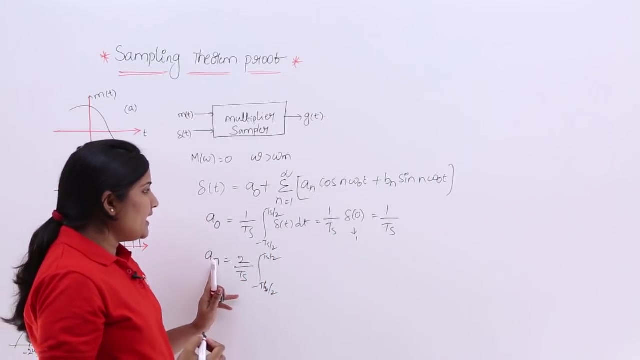 the sampling frequency. I am indicating sampling time period I am considering for impulse function. So 2 by t s integral, minus t s by 2 to t s by 2.. So here you are having a n value. a n is the coefficient of cos n. omega naught t, del of t into cos a. 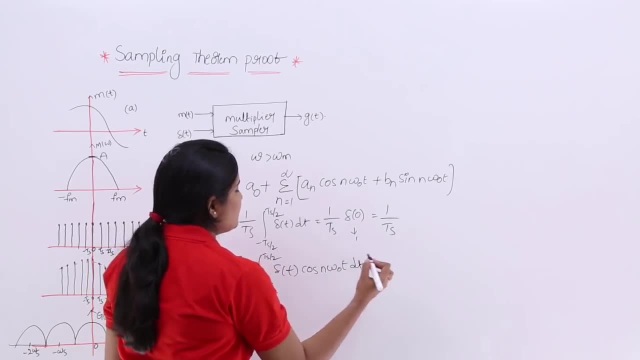 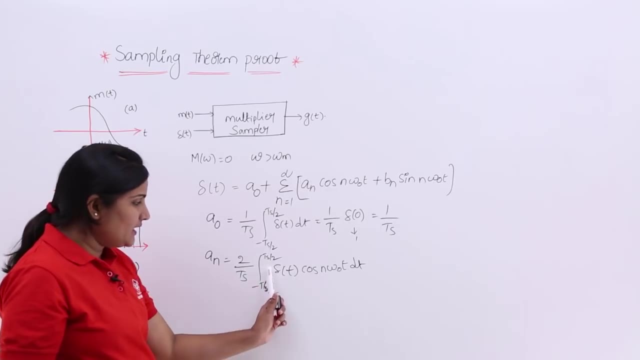 So cos n, omega, naught t. you need to write. So this is the equation for your even component. even component is equivalent to 2 by t integral your function, which we are representing in trigonometric series, into that even component. So cos n, omega, naught t, dt. So here also. 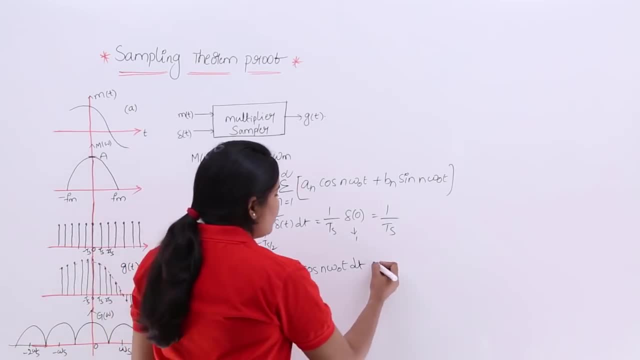 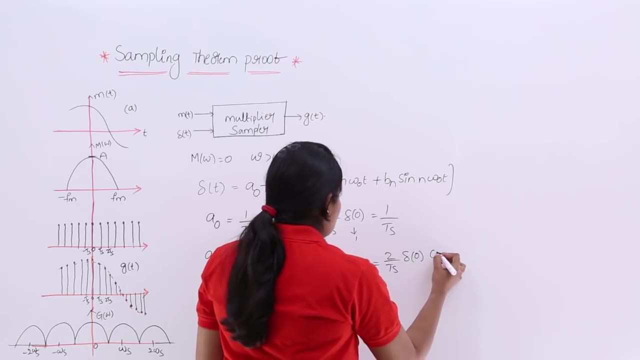 as you are having del function in integration, no need to integrate just you just write like this: That means cos n omega naught t del of t into cos a. So this is the equation for your even component del of 0: cos n omega naught into 0.. As cos 0 is equivalent to 1 and del. 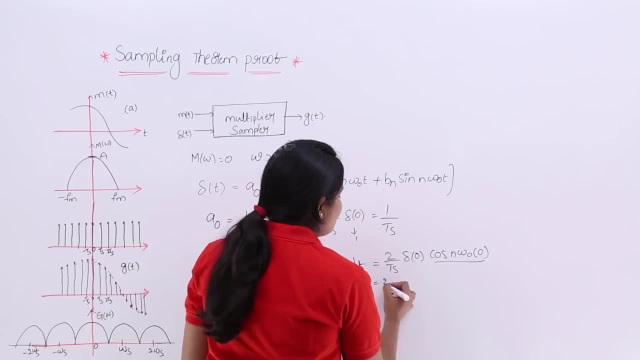 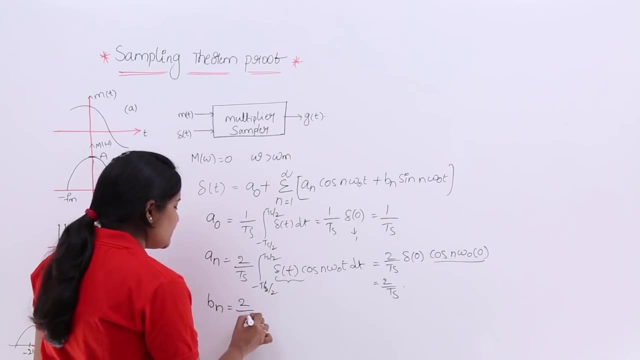 of 0 is equivalent to 1. your value is equivalent to 2 by t s. here Now coming to B n equation: B n is equivalent to 2 by t s, integral minus t s by 2 to t s by 2.. So in standard equations, in place of t s you are having t, So why I am taking 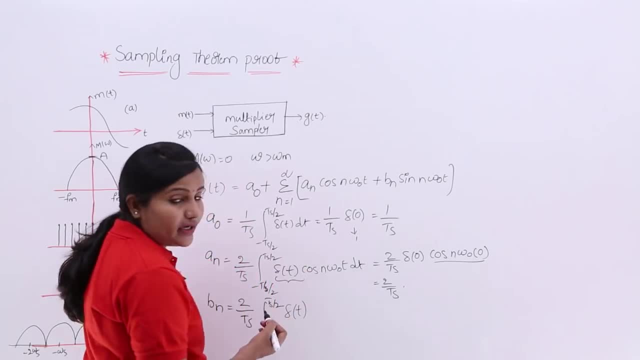 t s means Here my sampling time, frequency time period is equivalent to t s. So same equation. but as we are deriving odd component, odd multiplication factor, you need to write here: sin n, omega naught t dt Here. here also, you are having del of t in integration. no need to integrate. 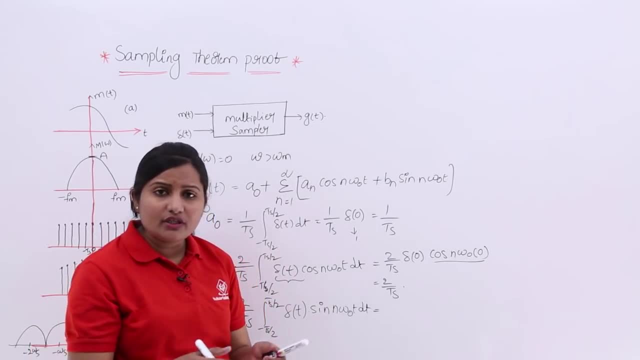 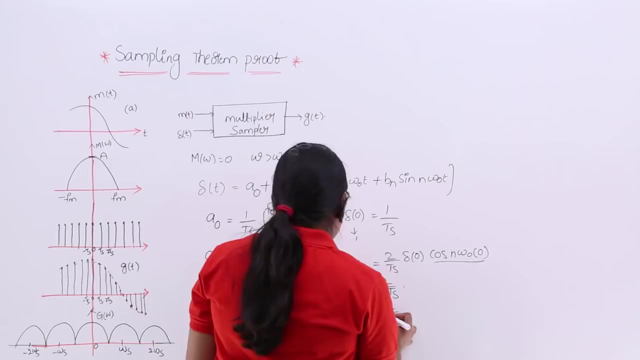 whenever you saw del of t in integration, no need to integrate why? because del function is only valid at a. t is equivalent to 0. Now you are doing the same thing in this standard equation, So you will get 2 by t. 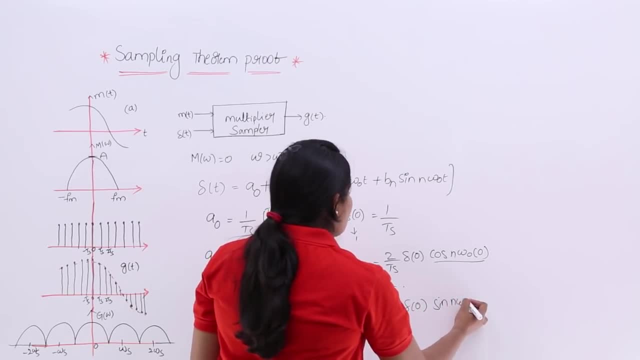 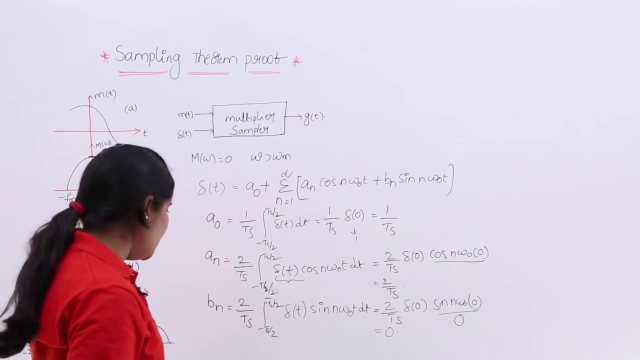 s into del of 0, into sin n, omega naught into 0. sin 0 is equivalent to 0, 0 into anything you are going to get 0 only. So now I am going to substitute all these values in this standard equation to get actual trigonometric Fourier series. representation of your impulse. 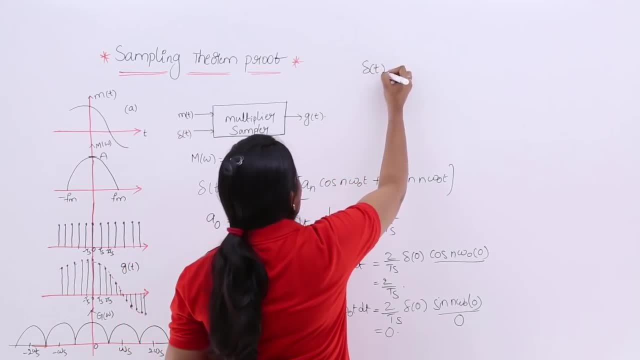 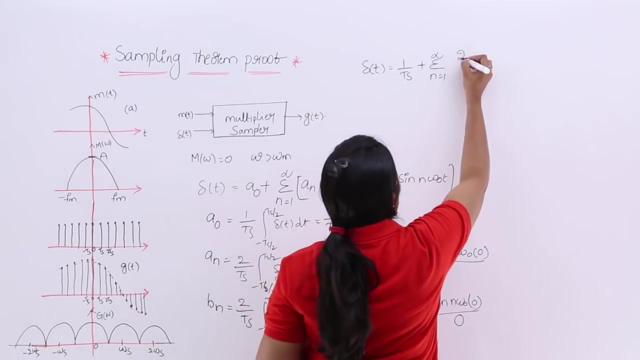 strain, So impulse strain. now, del of t is equivalent to 1 by t s, 1 by t s equal to 0. plus summation n is equivalent to 1 to infinity. summation n equivalent to 1 to infinity. in place of a n I can write 2 by T s, 2 by T s. cos n omega naught t, no need to have b? n value. 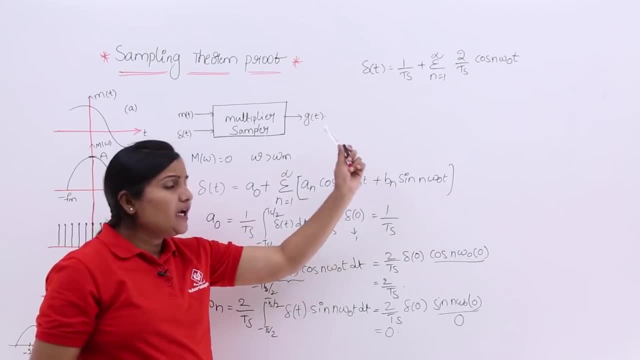 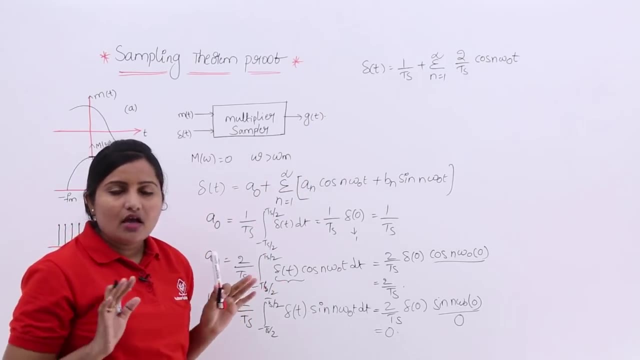 why? because b, n is 0, 0 into sin n, omega naught t, it will become 0.. So now you got trigonometric Fourier series representation of del of t. I am having my trigonometric Fourier series representation for del of t. if I am having trigonometric 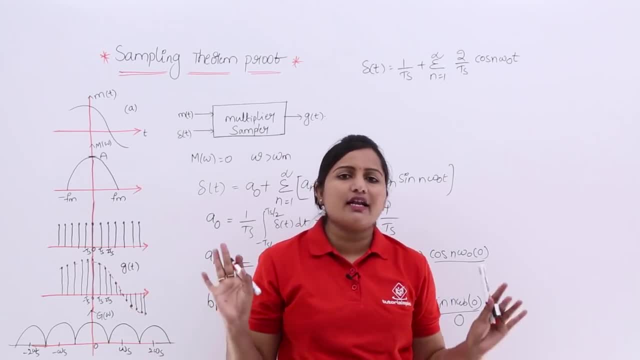 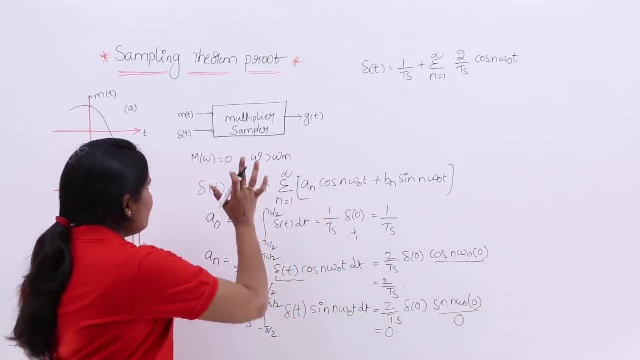 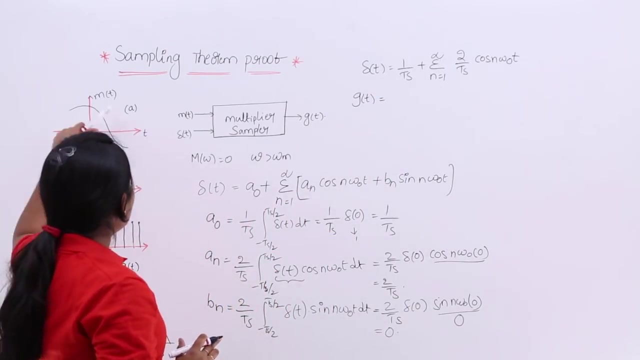 Fourier series representation. that means I am having value for del of t. I am. I described del of t with trigonometric coefficients, So here I am just applying this. so g of t is nothing, but now we are doing sampling. sampling means we need to multiply m of t with impulse. 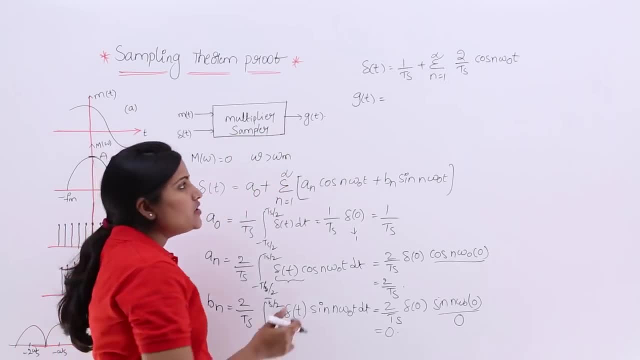 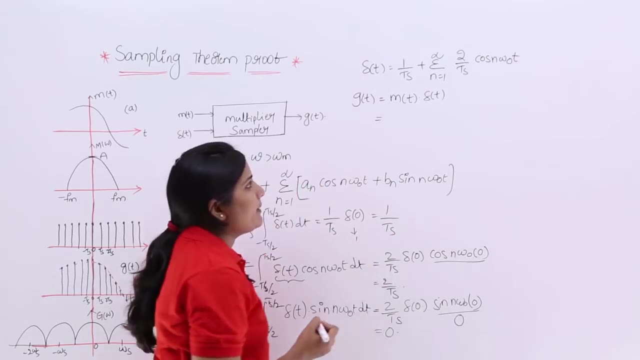 train you are going to get sampled signal g of t. So this is the sample Sampled signal which will come by multiplying m of t with this del of t. if you are multiplying m of t with del of t, so that means you are just multiplying m of t for this. if you are. 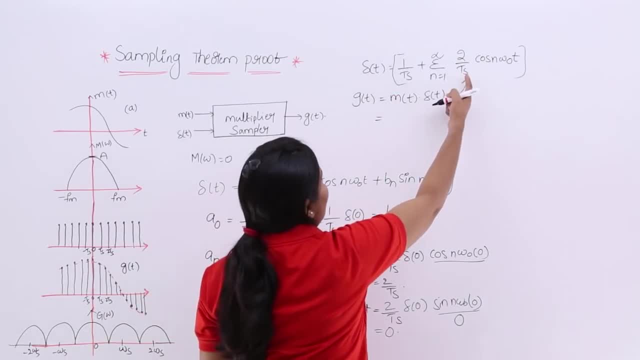 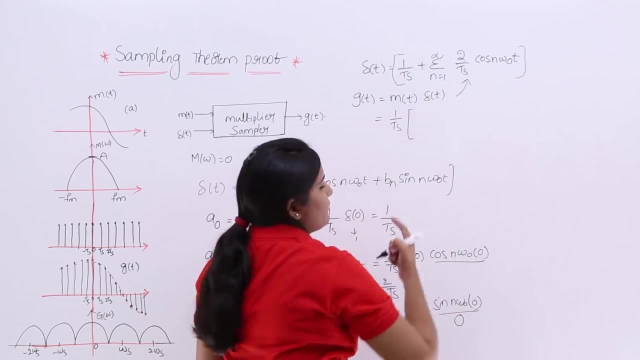 multiplying m of t for this. I am just writing like this: I am taking 1 by T s as common, 1 by T s as common. remaining is 1 plus summation 1 to infinity. 2 cos n omega naught t. for that I am multiplying m of t. 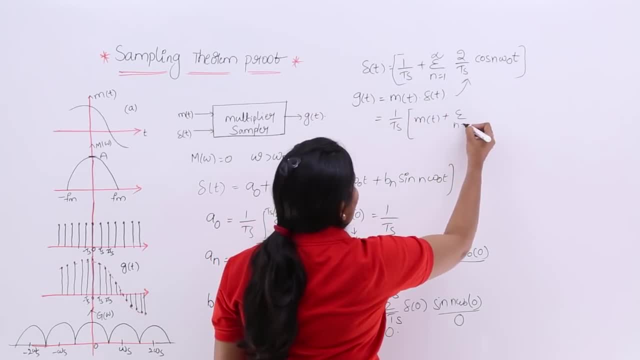 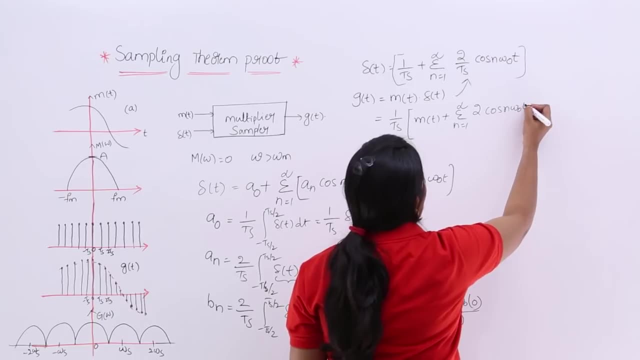 So m of t plus summation n is 0. So m of t is equal into 1 to infinity. so here you are getting 2 cos n, omega naught t. So like this you are getting. so now, in the next step, I am going to consider like this: 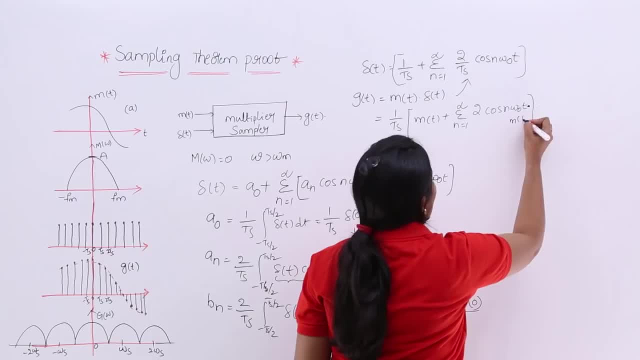 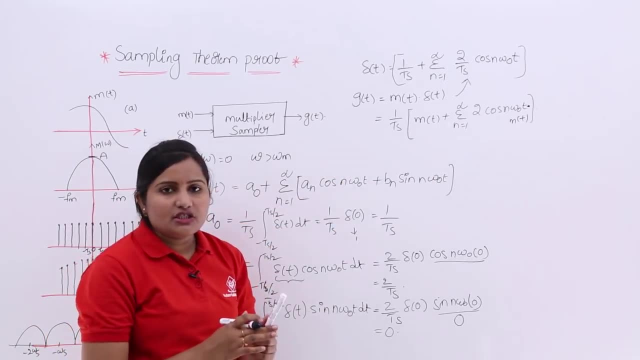 2 cos n. omega naught t into m of t. this m of t can be multiplied here and here. So now you can see, if you consider that summation as extended summation, then how you are going to get you can. you can observe. 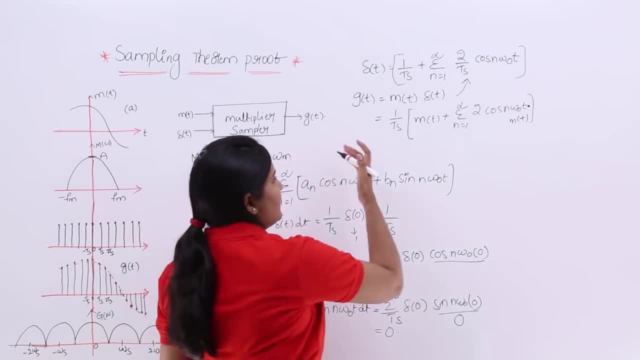 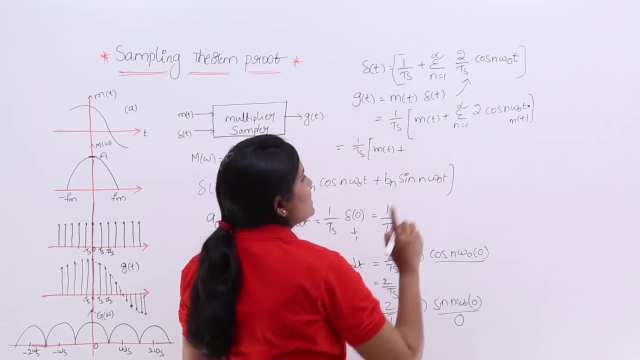 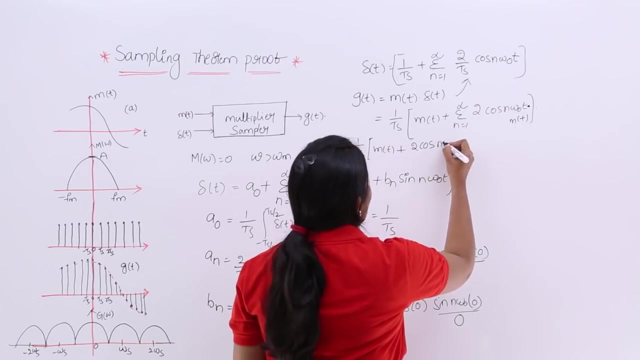 How you are going to get your extended summation- means that is equivalent to 1- by T s, m of t plus. if n is equal to 1, what will happens? if n is equal to 1, that is equivalent to 2 cos. if n is equivalent to 1, you are going to get cos omega naught t into m of t plus. 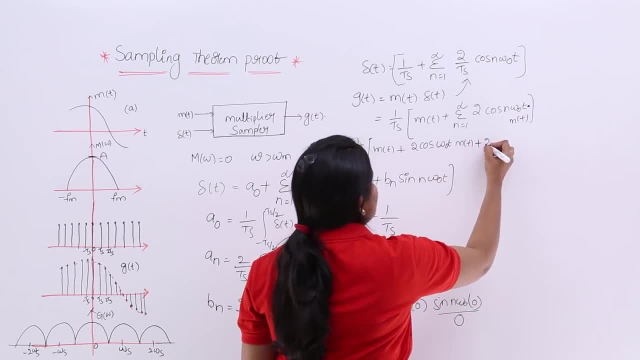 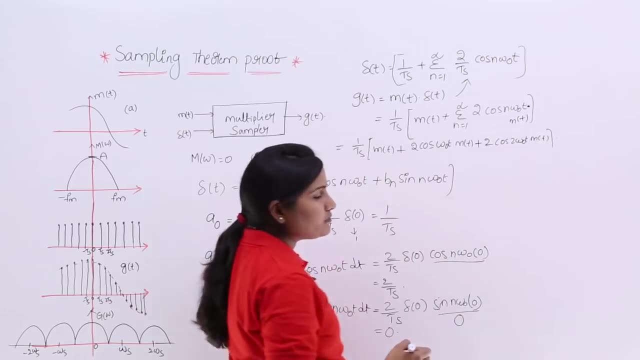 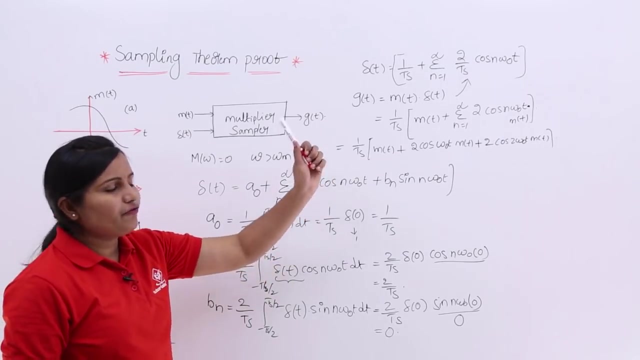 If n is equal to 1.. if n is equal into 2 cos 2 omega naught t into m of t, like that you are going to get. So now, if you observe- here I am considering g of omega- how we will get g of omega. So 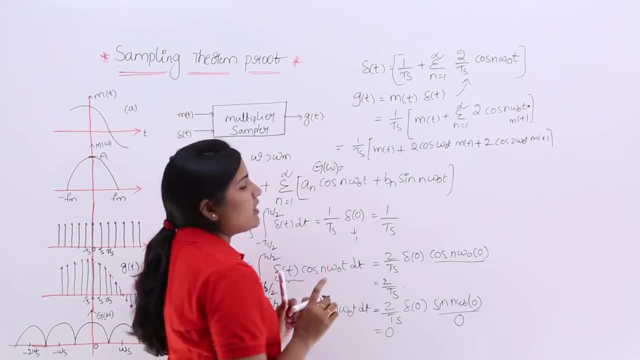 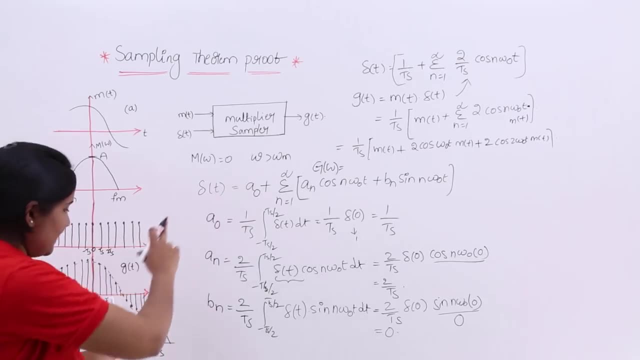 g of omega means considering transform of g of t by just considering the Fourier transform of g of t. this is sampled signal. that means that is the equation for this signal. So and we need to get the equation for this spectrum. So if you want spectrum of this sampled signal, 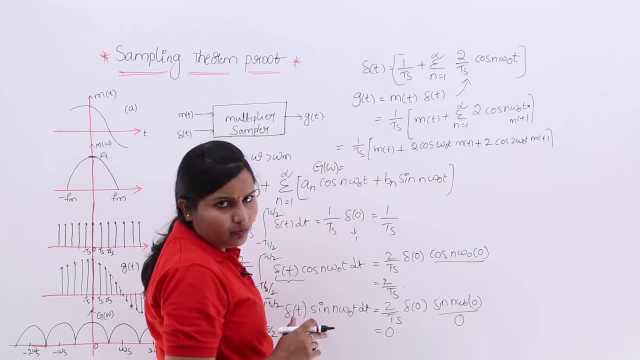 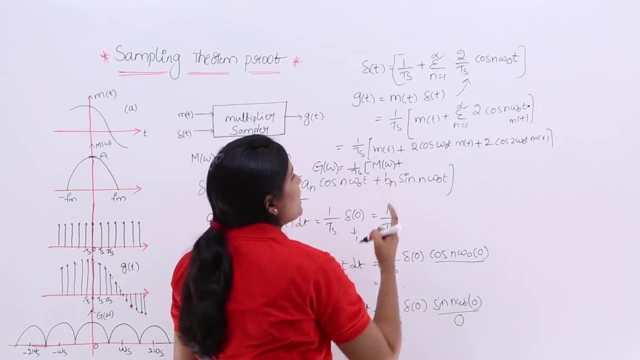 so then we need to consider Fourier transform on both sides, then you will get 1 by t s. So here you will get m of omega plus here you are having cos omega naught t, I will tell you for one thing. So you are having 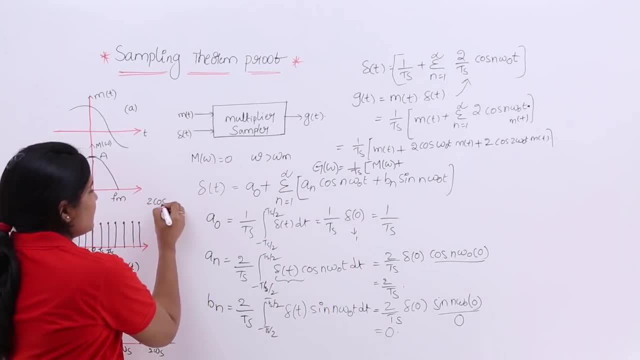 So you are having cos omega naught t, 2 cos omega naught t, this 2 cos omega naught t. how you can write So 2 into e power minus j omega naught t plus e power minus e power plus j omega naught t, divided by 2.. So 2, 2 will be cancelled in place of cos omega. 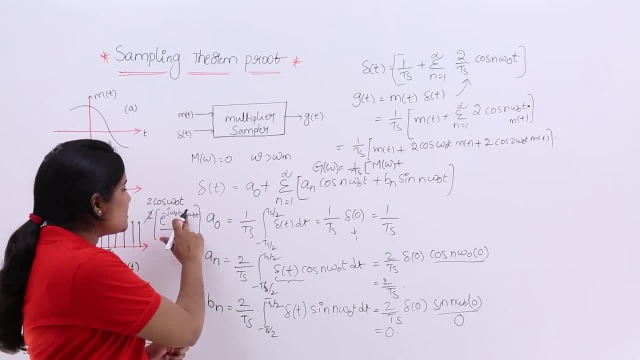 naught t. now onwards you can think: e power minus j- omega naught t plus. e power plus j- omega naught t. In place of 2 cos 2 omega naught t, you can write 2 cos omega naught t every time 2 is going to cancel, but in place of omega e power minus j, 2 omega naught t plus. 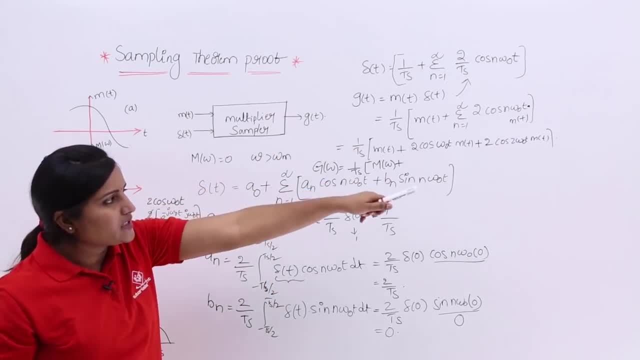 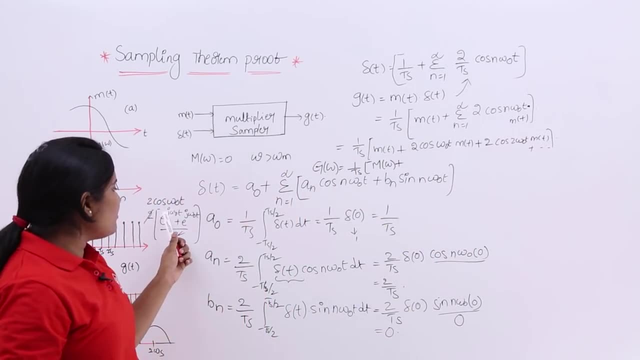 e power, j, 2 omega naught, t in case of next term. So this is a summation, So so, on so many terms will be there. So in next term you are getting e power minus j, 3 omega naught. 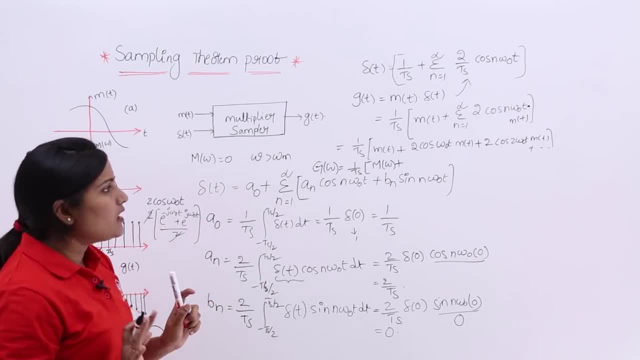 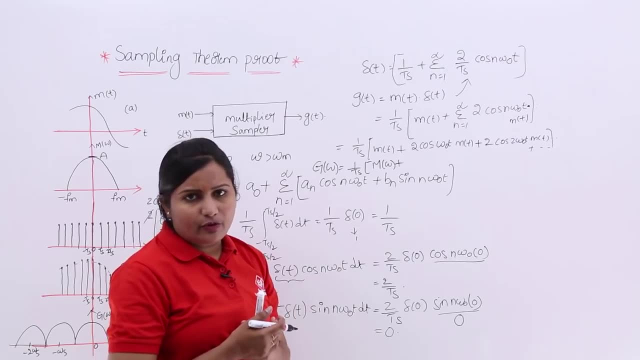 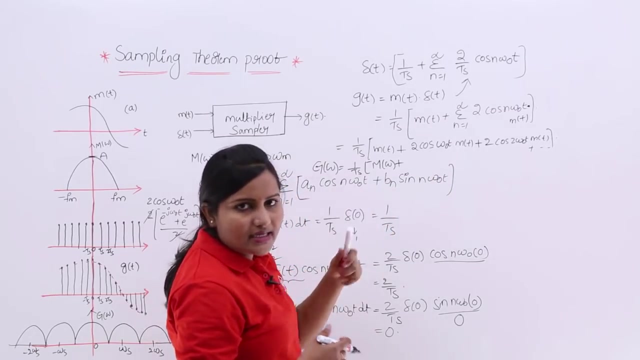 t plus e power plus j, 3 omega naught t like that. So you are having frequency shifting property. You are having frequency shifting property. So how frequency shifting property will work For m of t if m of m of omega is the 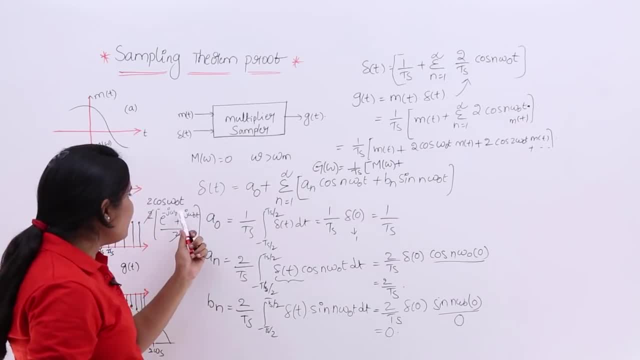 transform, then e power j omega naught t into m of t is having transform of m of omega minus omega naught and e power j omega naught t into. So for this you can see, if m of t is having transform m of omega, then what will happens. 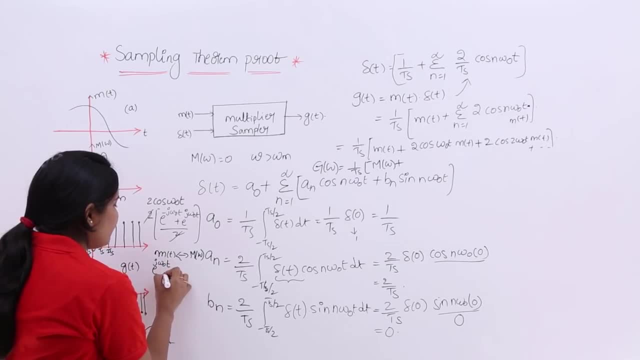 If you consider e power minus j 3 omega, naught t plus. e power plus j 3 omega, naught t plus. e power minus j 3 omega naught t into m of t. So frequency shifting property in Fourier transform m m of omega minus omega naught. If you consider e power minus j 3 omega naught. 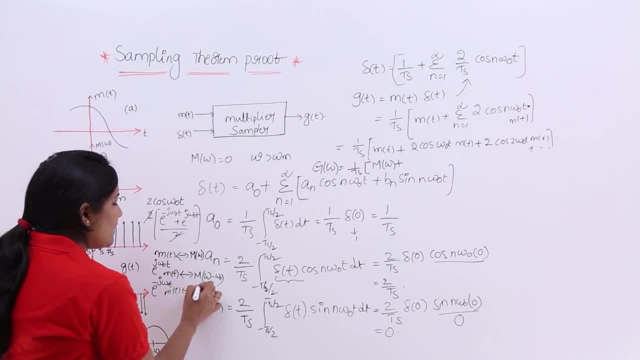 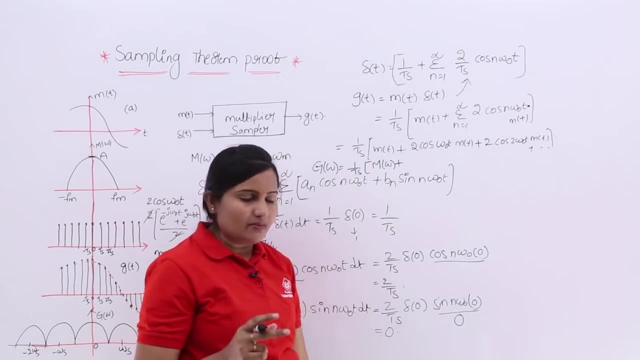 t into m of t. what will happens? So m of omega plus omega naught. that means for each cos we are going to apply frequency shifting property 2 times, that means because of multiplying e power- j 3 omega naught t. e power minus j 3 omega naught t to this m of t. I am going 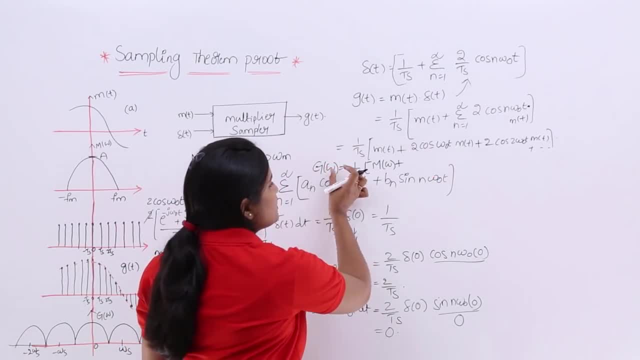 to apply frequency shifting property 2 times. that means because of multiplying e power j 3 omega naught t. e power minus j 3 omega naught t to this m of t. I am going to apply f over this m of t. I am just using transform. I am writing transform In this place. I am 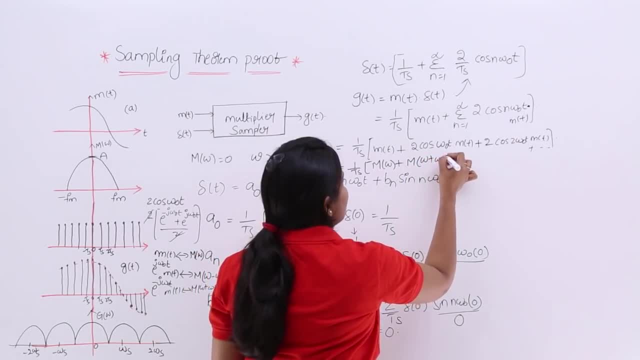 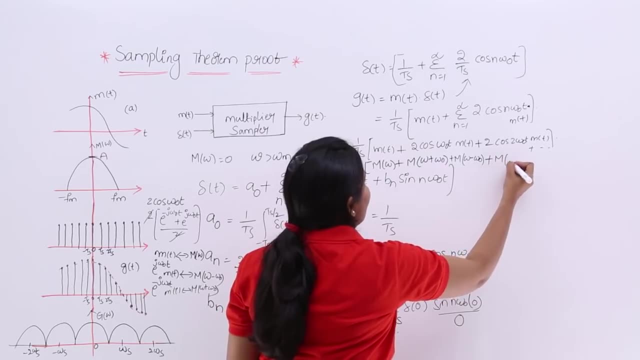 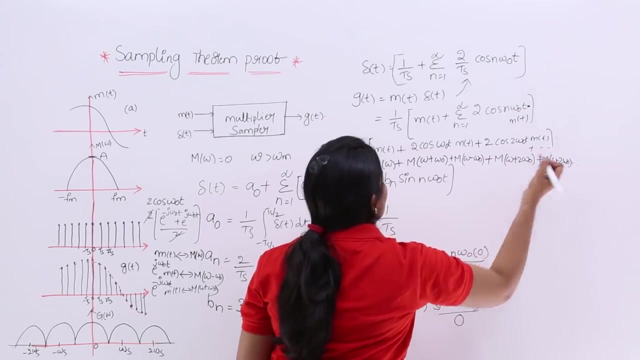 going to write m of omega plus omega naught plus m of omega minus omega naught, So plus. in this place I am going to write m of omega plus 2 omega naught plus m of omega minus 2 omega naught. like this I am going to write: So everything I want to write, like this: j. 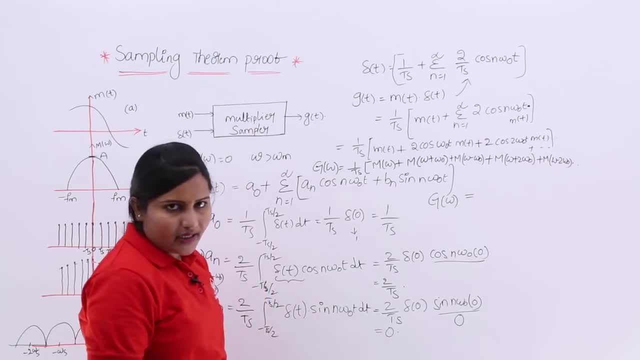 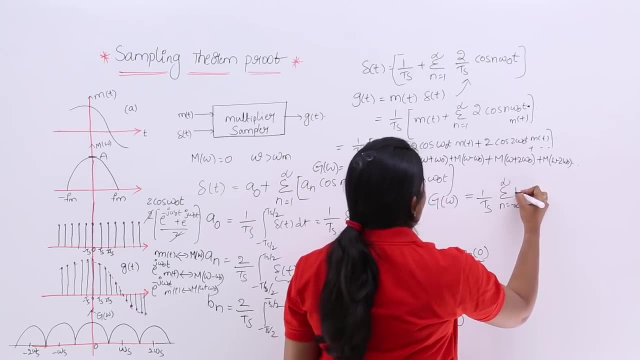 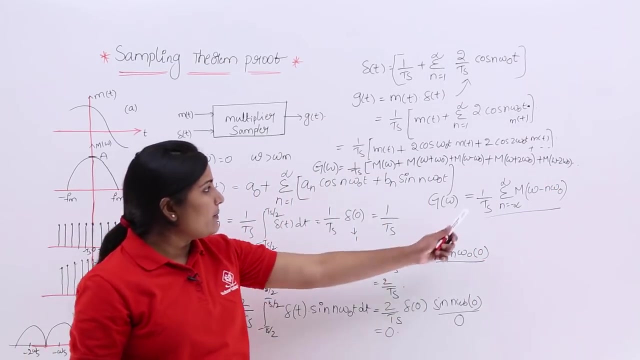 of omega is equivalent to. So this is the truth. So if you consider e power plus j, equivalent to G of omega is equivalent to 1 by T s summation, n is equivalent to minus infinity, to infinity. m of omega minus n omega naught, I am writing like this: finally, 1 by 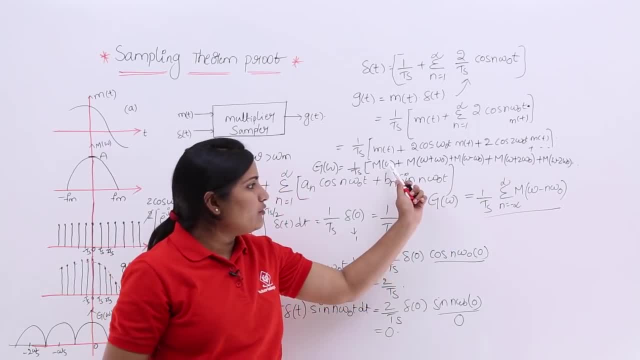 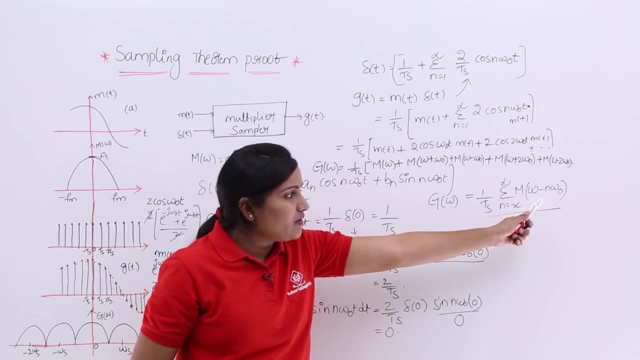 T s into. So everything I included omega naught as 0. n is equivalent to 0 term. if n equivalent to 0 m of omega will come. if n is equivalent to 1 omega minus omega naught will cover n is equivalent to minus 1 omega plus omega naught will cover. So all that. 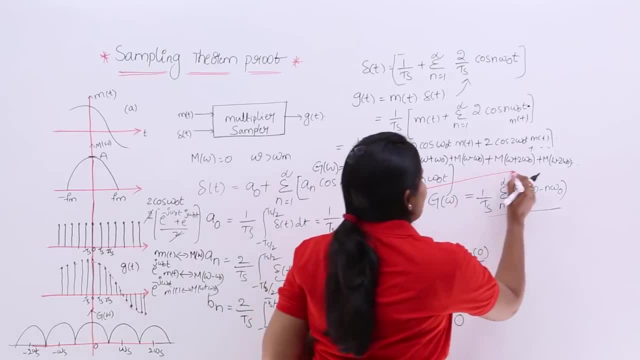 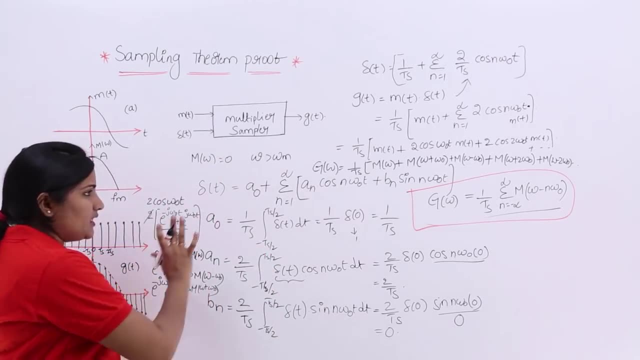 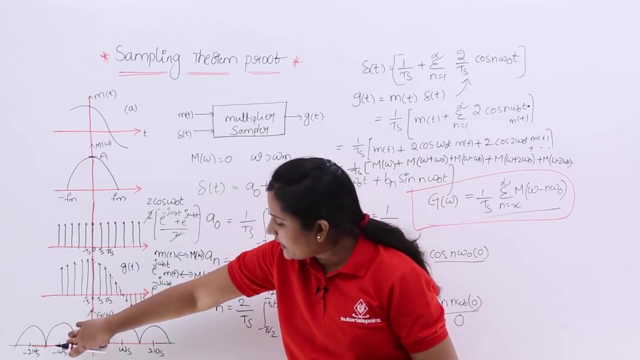 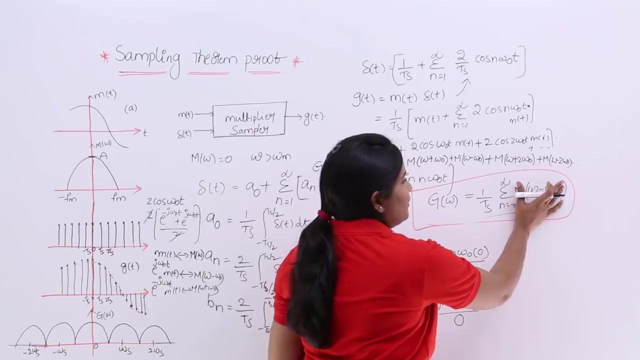 summation will cover in this equation. this is your spectrum of sampled signal. this is the spectrum of sampled signal. Now, coming to this spectrum of sampled signal, if you want to reconstruct your signal, you will pick a spectrum, you will pick a spectrum from here and you will take inverse transform. So in this, in this summation, you, you just 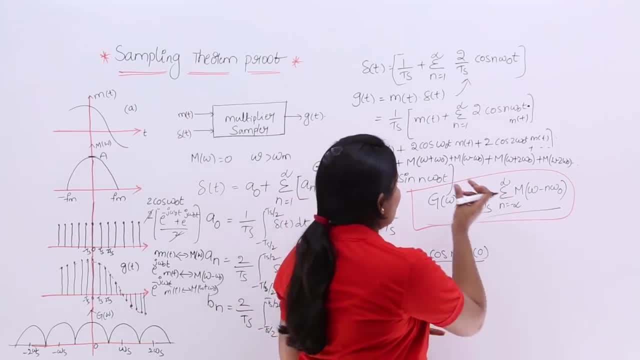 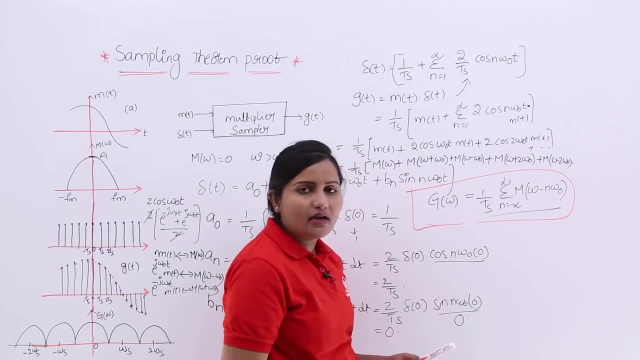 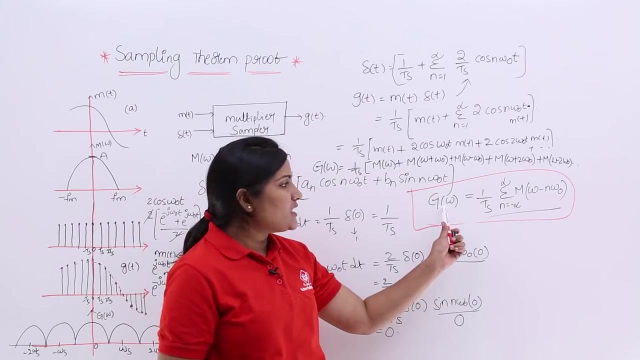 consider any m of omega. that means you can consider m of omega, or you can consider m of omega plus omega naught. you can consider m of omega plus omega naught. you can consider any spectrum, individual spectrum. you can take inverse transform if you consider inverse. 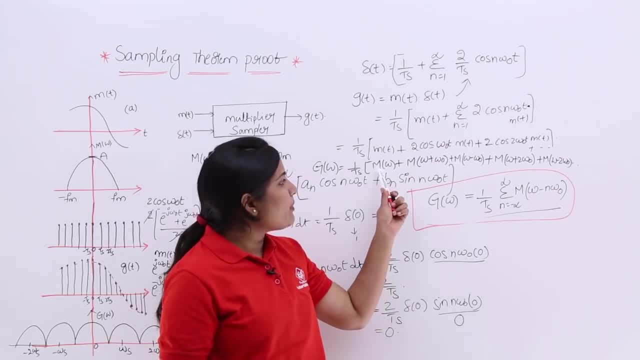 transform, you will get G of T. So if you consider m of omega, you will get G of T. If you consider m of omega plus omega naught, you will get G of T plus T naught, like that shifted version you will get. So you are going to get this signal, whatever it may. 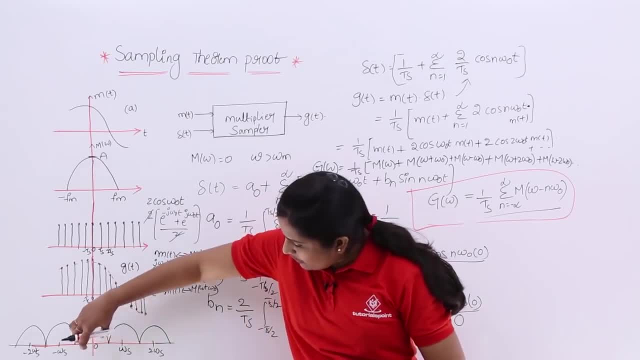 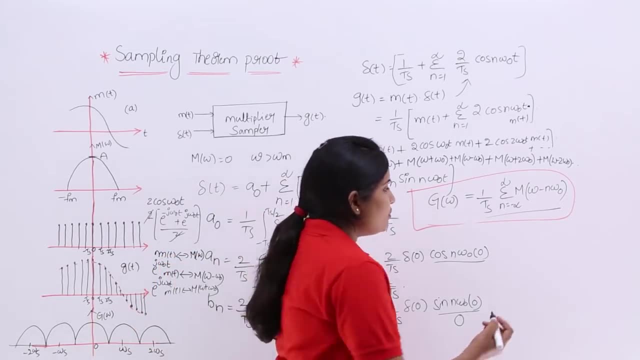 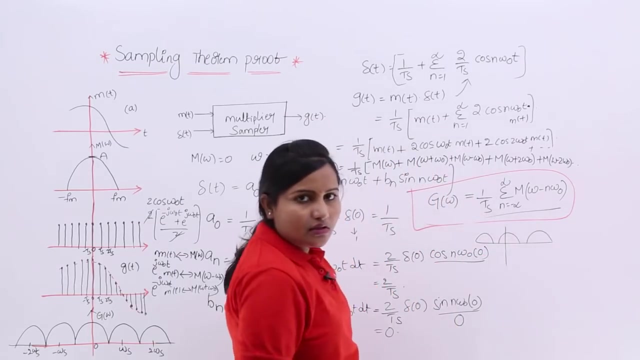 be. finally, you are going to get this signal by extracting any one of this spectrum and by taking inverse transform, you are going to get your signal back. So now coming to the conditions. so here, if this spectrum is like this, this is you. 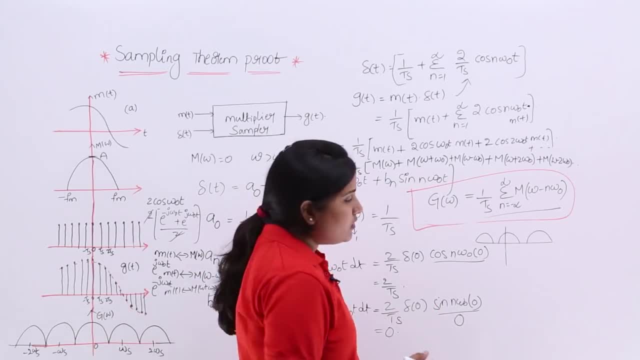 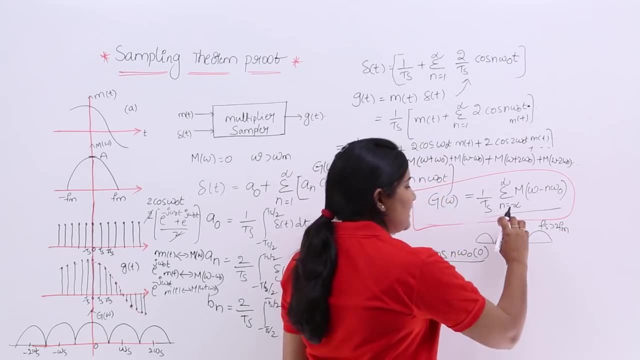 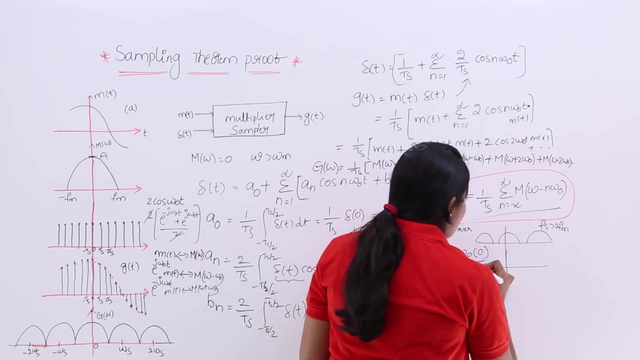 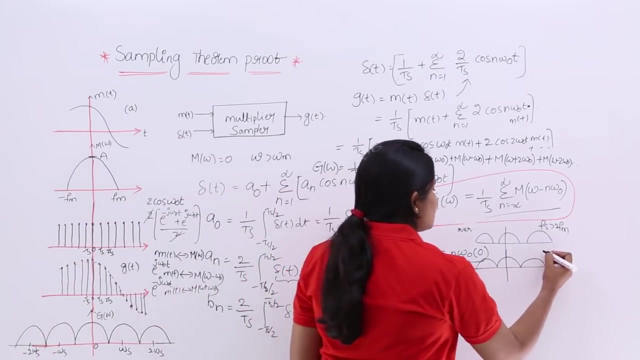 know this is O sampling. So here you are taking fs greater than 2 fm, So here you can easily pick any one of this spectrum. So here this is O sampling. So here another case is there. So like this: whatever we consider, this is the standard case. So this is perfect. 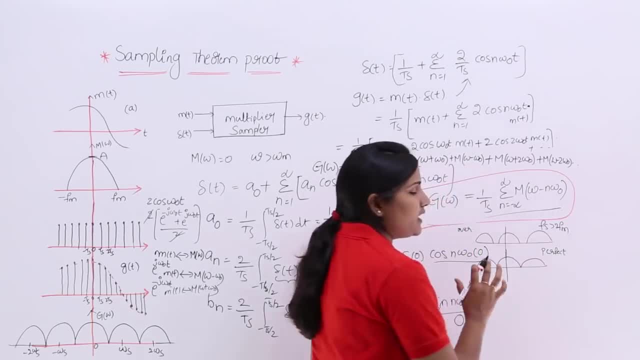 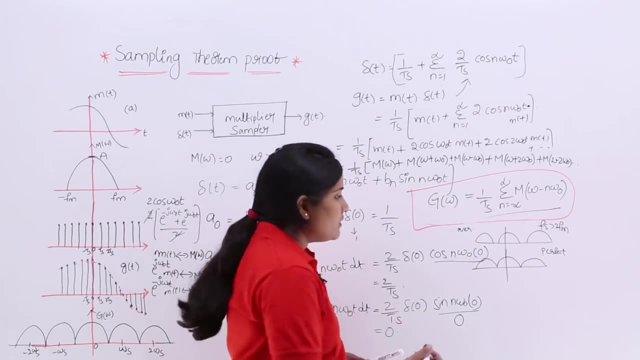 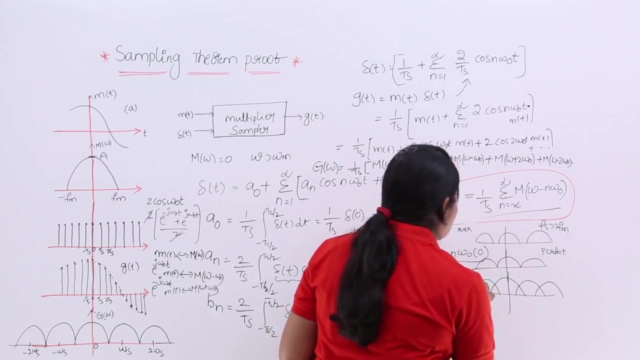 sampling, perfect sampling. here also we can consider samples, but we are not going to do that, But practically this is also not going to work. we are going to get crossed up, And here, finally, we are having another case that is under sampling. So under sampling means so if you consider fs, less than 2 fm. 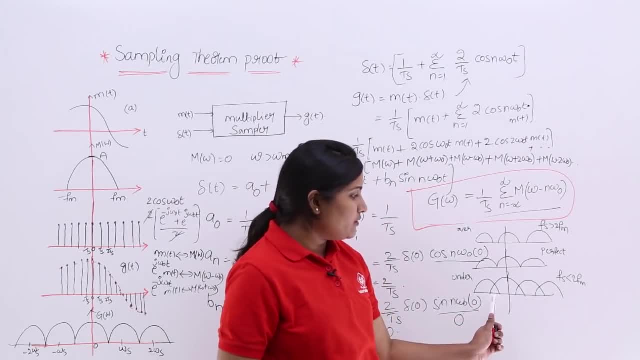 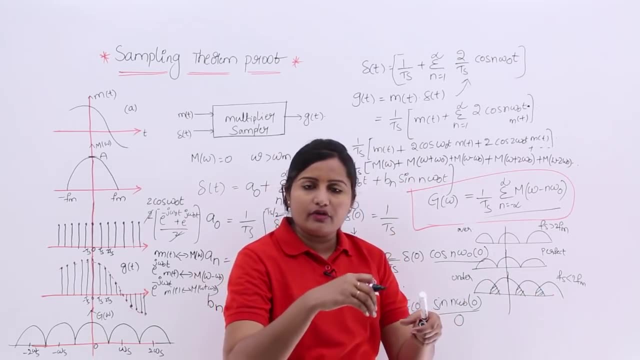 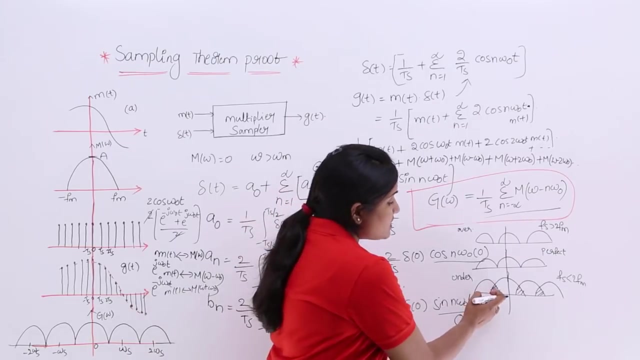 you are going to get your spectrum like this: you are going to get your spectrum with aliasing. that means your spectrums are going to align. you are going, your spectrums are going to combine. So in this case, what will happens? if you want to pick this spectrum, then some of the 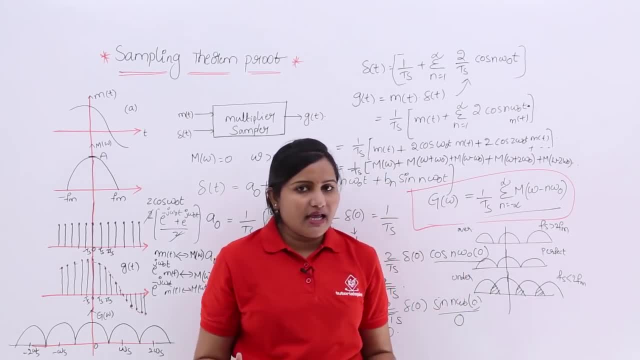 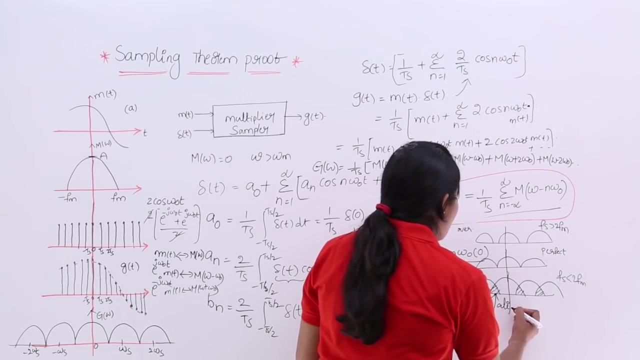 components of this spectrum is also coming, Then what will happen? So you will get components of other signal, that is, that will be a noise for your requirement. So this is called as aliasing effect. this effect- overlap of spectrums- is called as aliasing aliasing effect. So 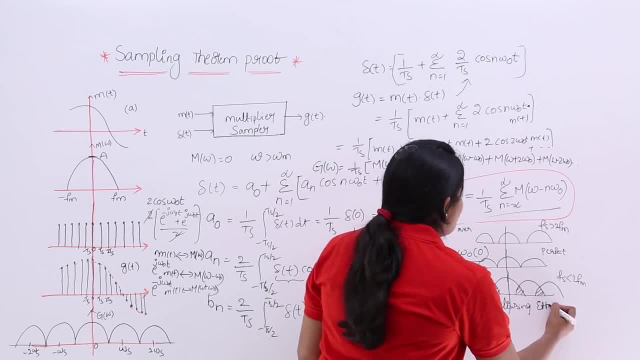 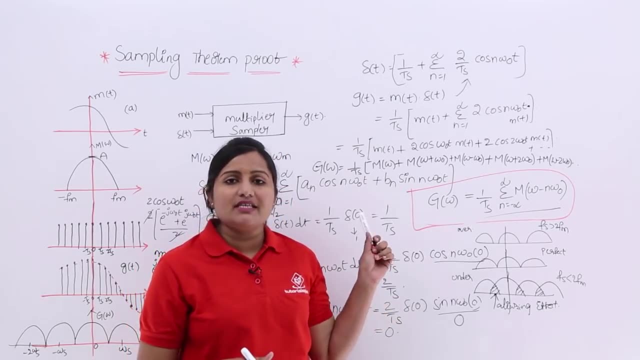 to reduce this effect. we need to reduce this effect. we need to reduce this effect. we need to use anti aliasing filters or we need to use fs greater than 2 fm. So best conditions are these two. if you consider fs greater than 2 fm, that is perfect to reconstruct your signal. 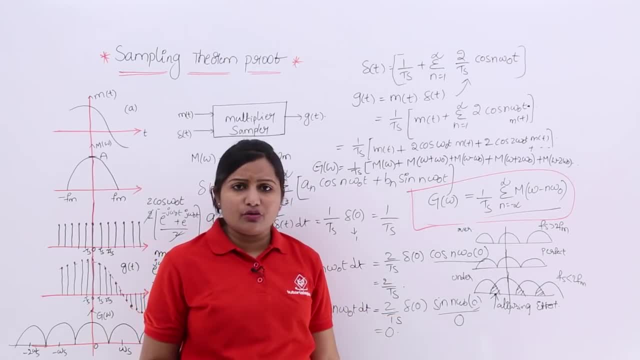 back. For example, if you are using fs less than 2 fm, if you are not using any GERD band, if you are not using any GERD band, this is the spaces in the spectra is called as GERD band. using got band, there are many chances for overlapping of spectrums and there are many 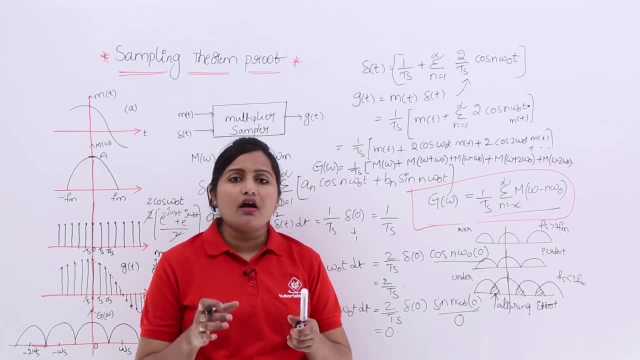 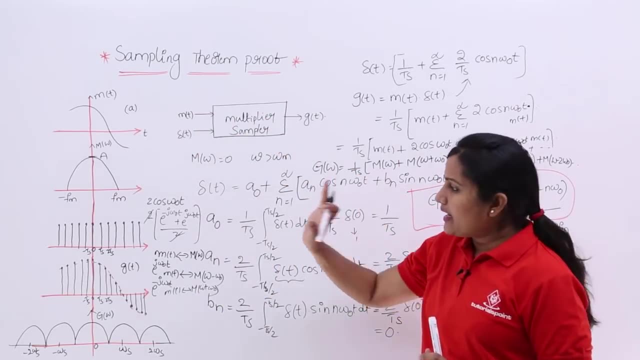 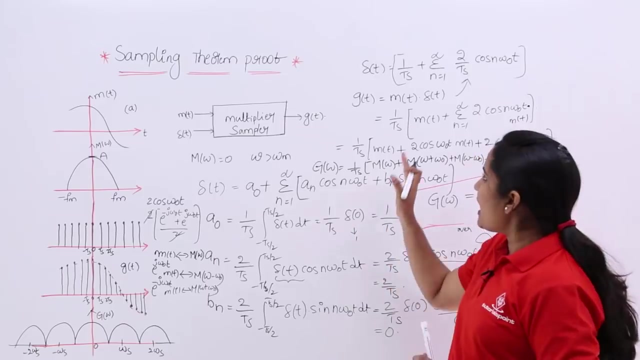 chances that you will get noise in u o output signal. So what we are doing is, finally, I will tell you. So I consider a signal, I consider a impulse time. So I given representation of impulse time for multiplication. So I multiplied. 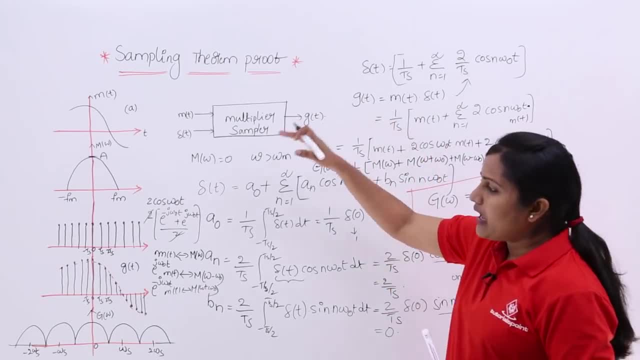 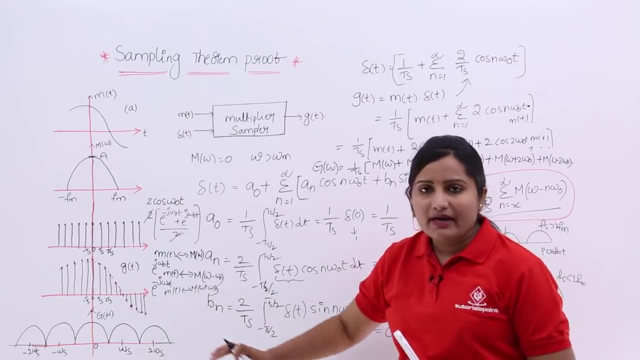 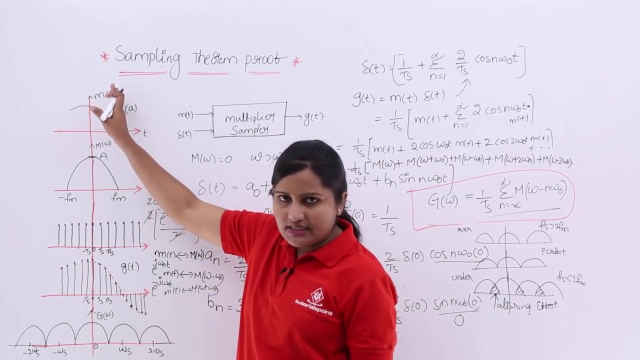 my message: signal with impulse, and here I consider the spectrum of sampled signal. So I consider spectrum of sampled signal in that spectrum. why I consider spectrum of sampled signal? So here envelope will shows you this signal. but practically to reconstruct the signal from the sampled signal you need to consider the spectrum of sampled signal. and 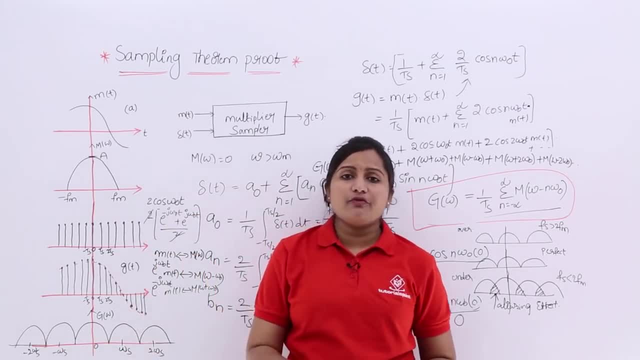 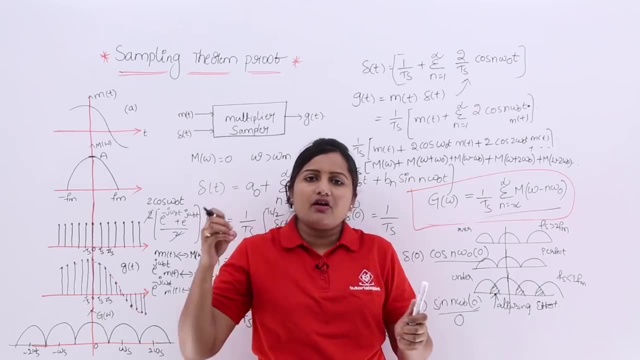 you need to pick a spectrum, you need to take inverse function of the signal, So inverse Fourier transform of that spectrum. you will get G of t again. That means in this summation you can consider any one of that spectrum of M, of t and you need to consider: 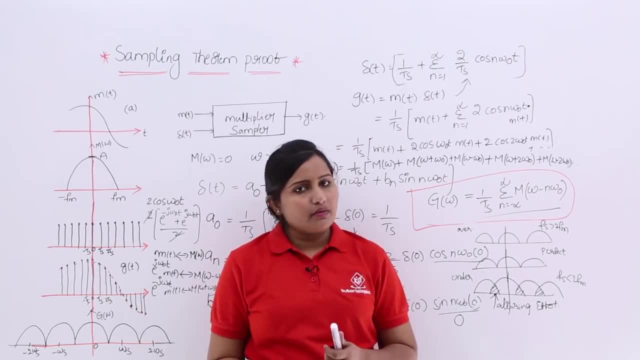 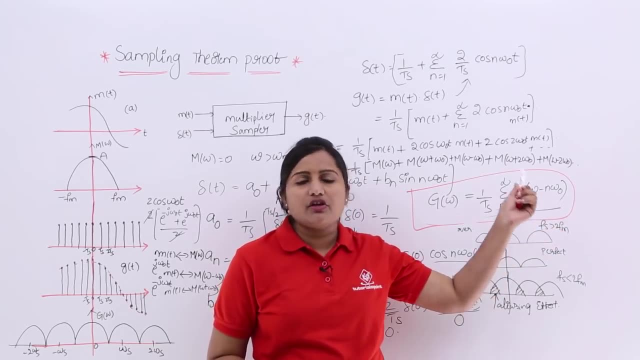 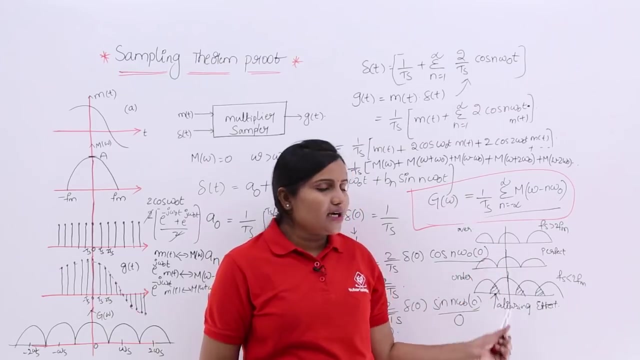 inverse Fourier transform to get you a M of t. So in this M of omega, if you consider, you will get G of t. if you consider shifted spectrum also, you are going to get shifted version of your signal. same M of t signal you are going to get. So here, these are the 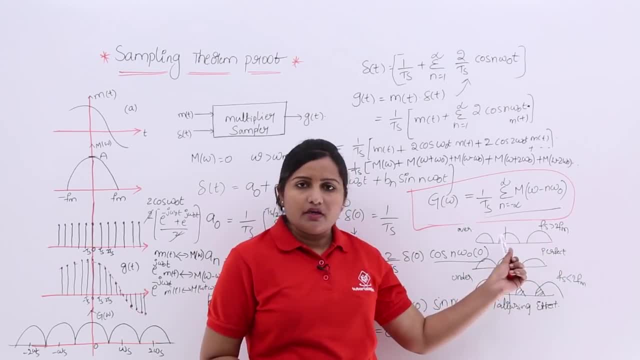 conditions. So if you consider fs greater than 2 fm, picking of spectrum is easy. here is also somewhat ok. but if you consider that means this is under sampling, under sampling, aliasing effect will come. to reduce this aliasing effect you need to consider your sampling frequency, fs. 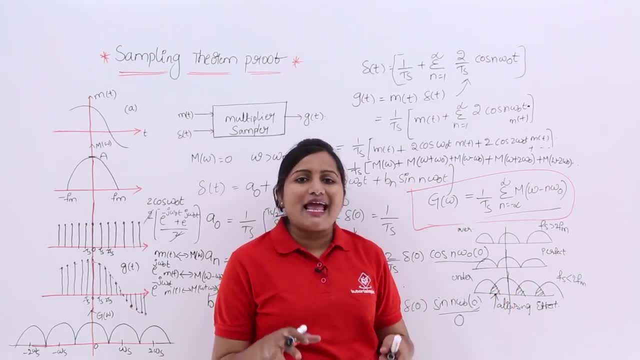 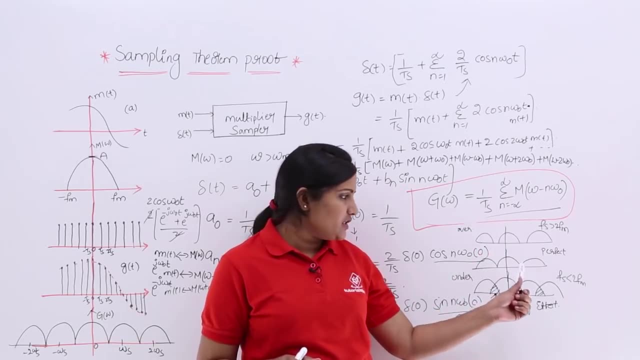 greater than 2 fm or you need to use anti aliasing filters. So the best condition is fs greater than 2 fm, condition over sampling condition and perfect sampling condition is greater than 2 fm, So perfect sampling condition is also somewhat ok. that came by considering Nyquist trait. 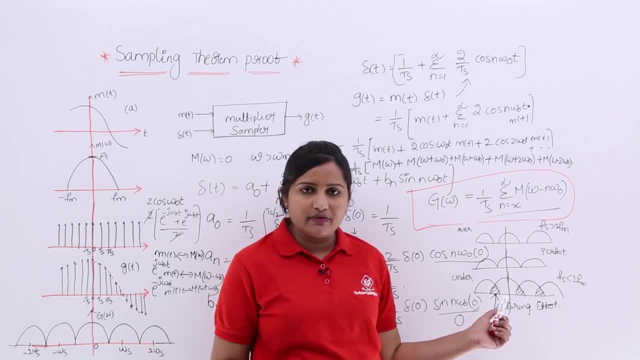 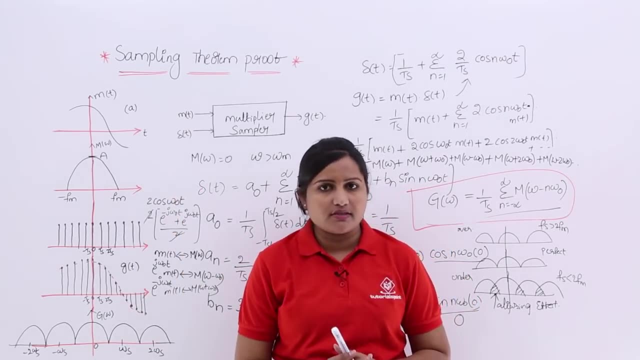 but this condition is not perfect. it will get aliasing effect. you need to consider aliasing filters. ah, again, if you consider this case when you are doing this process. 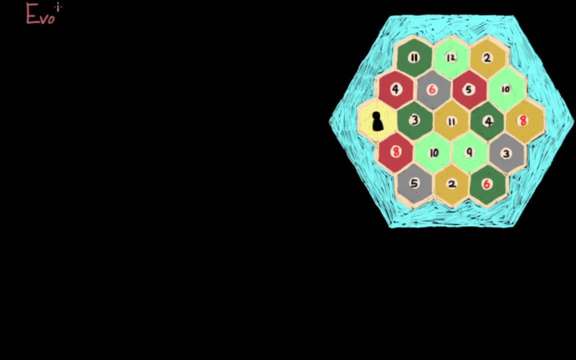 Game theory is usually talked about in reference to decision making, but we can also use it to talk about evolution and animal behavior. But before we do that, I want to take a moment to talk about how game theory is usually discussed. So when I think about game theory, I generally think about it as it relates to the social sciences, or maybe economics. 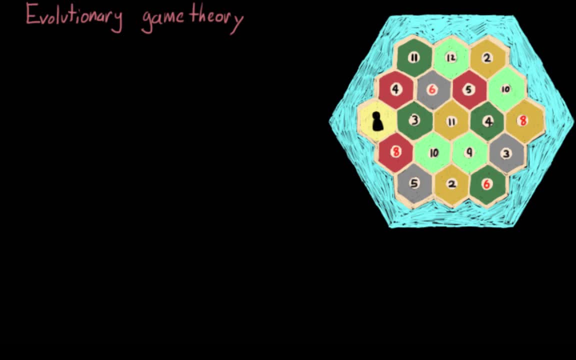 But we can also use it to talk about everyday behavior. So imagine that we're watching a group of people play a game, an actual board game, like maybe Monopoly or Settlers of Catan. The individuals who are playing these games make decisions like whether or not to put a settlement on a wheat field. 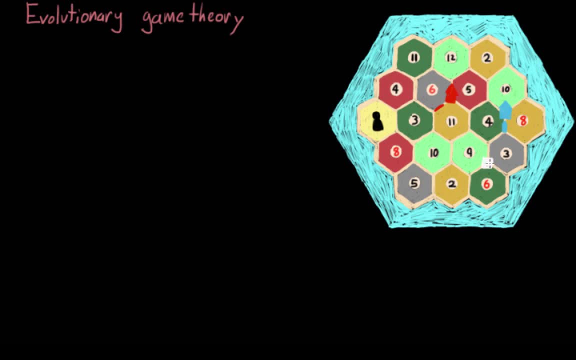 But the results of that decision don't only affect that individual player. It affects everyone who is playing the game. So the playoffs to each of the players depend upon the decisions made by the overall group. And this is where game theory comes into play, because it reasons about and tries to predict the behaviors that we would expect to see when the individuals are playing this game. 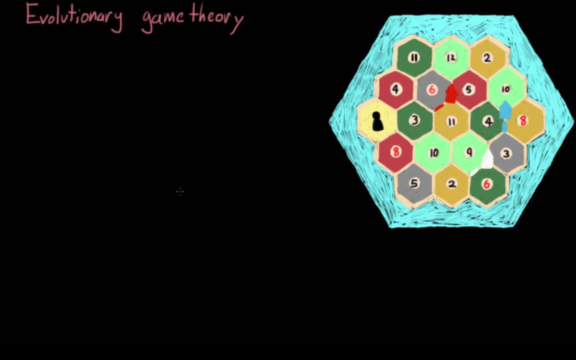 So, while it looks at things like individual strategy, it also looks at how we reason about what the other players are going to do, Like the training, Like the trades that they're going to make, Or whether or not they'll go for longest road.